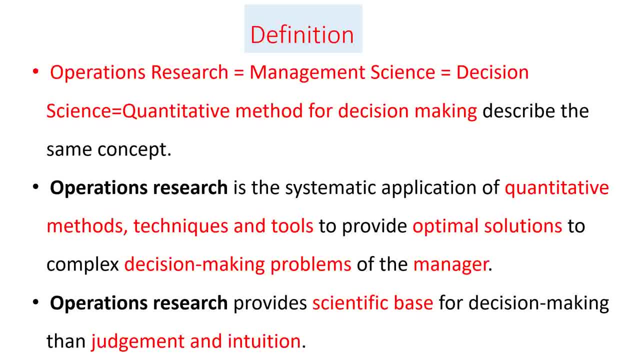 For example, operation research, management science, decision science, quantitative method for decision making, describe the same concept. In our discussion we will use the term operation research. In the organization we know that there is a conversion of input to the output. That's called operation. 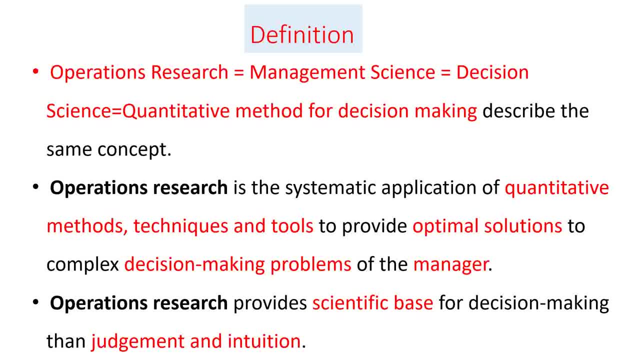 And a manager is expected to be efficient in the allocations of such resources or factor of production so that the company can maximize the output or minimize the cost as much as possible. An important activity of a manager to bring this optimization to the table is the implementation of operational research. 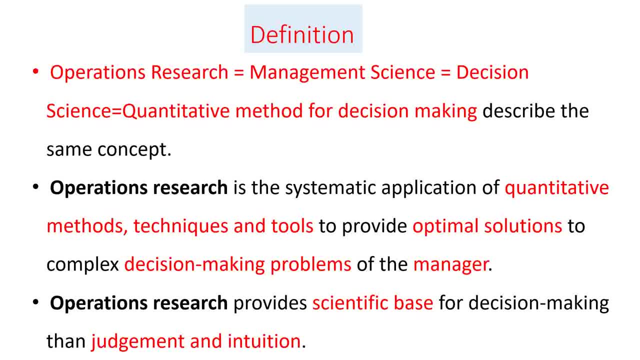 The first objective of operation research is to make well and informed decisions. Indeed, a manager in the organization can use his experience, judgment or intuition, or we can say in short, qualitative data and quantitative methods, to make better decisions. Thus, from this, we can understand that operation research is a scientific system. 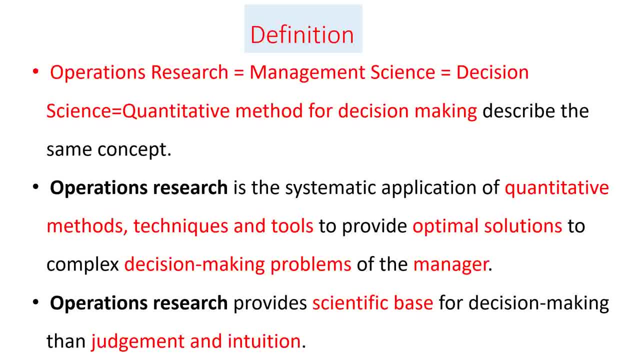 The second objective is to make well informed decisions. The third objective is to make well informed decisions. The fourth objective is to make well informed decisions. Thus, from this we can understand that operation research is a scientific system. Thus, from this we can understand that operation research is a scientific system. 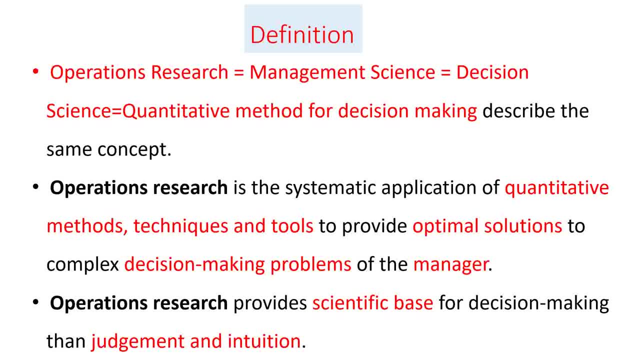 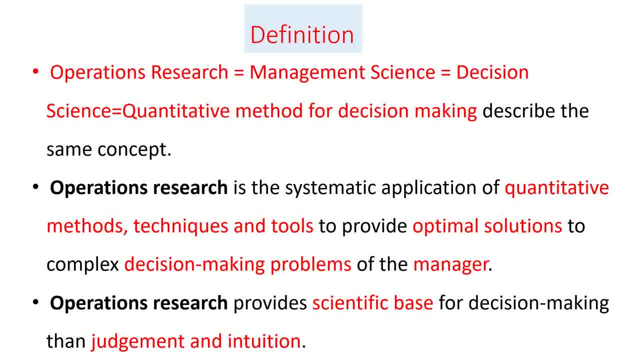 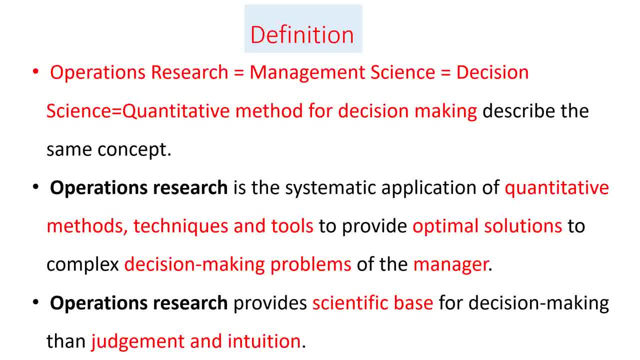 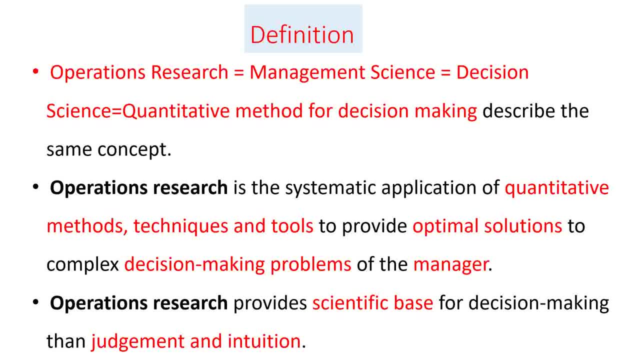 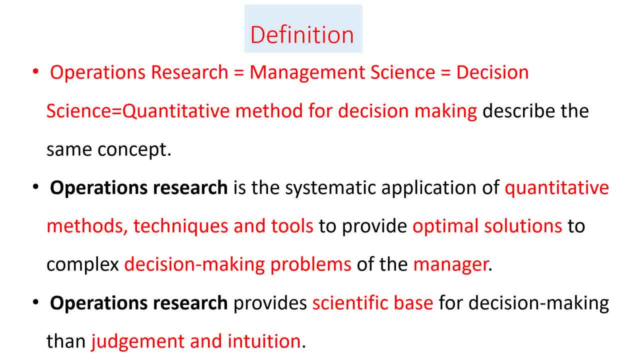 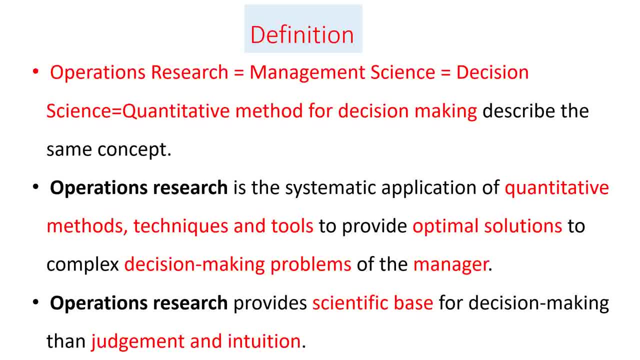 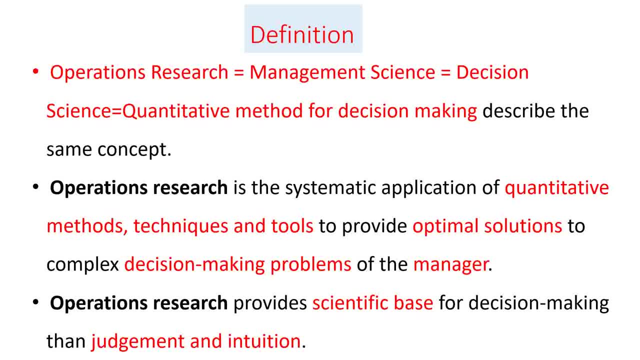 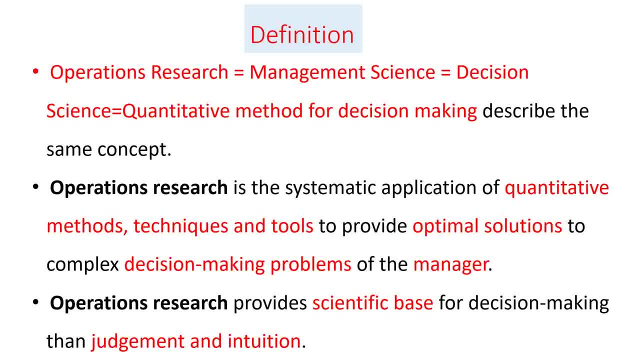 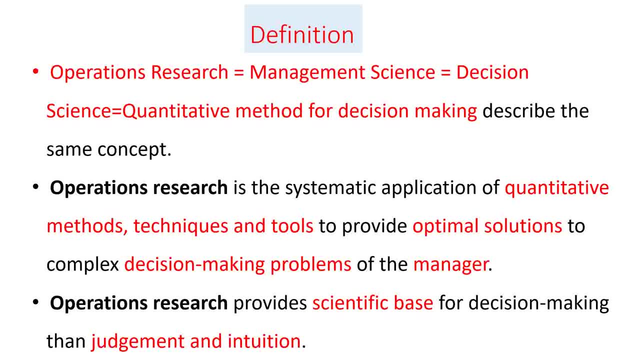 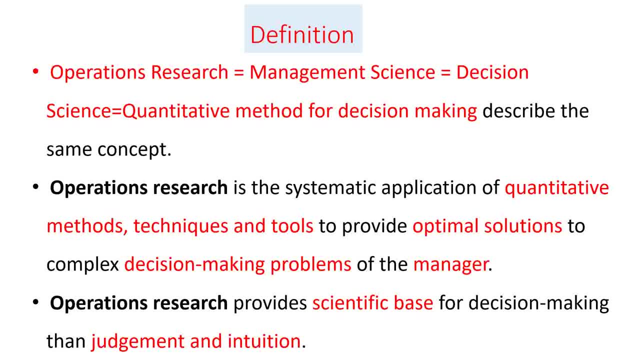 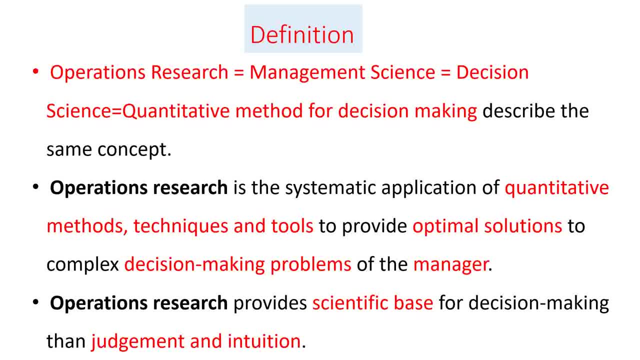 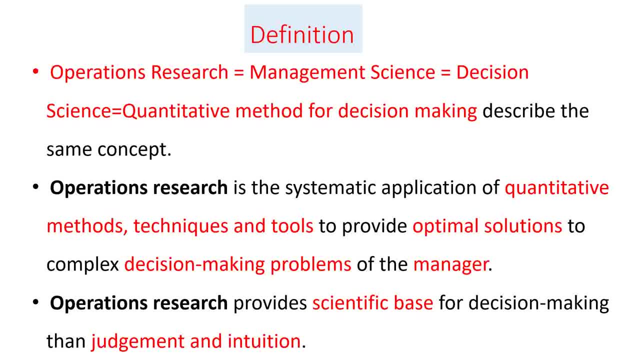 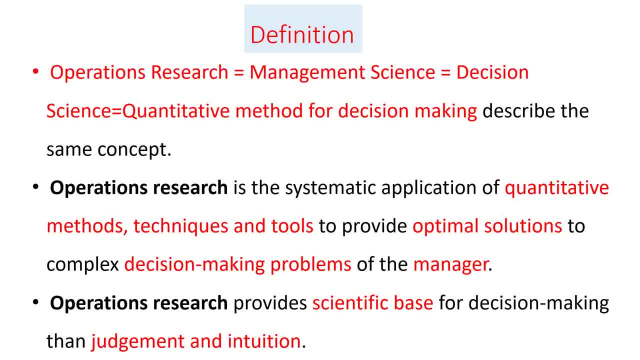 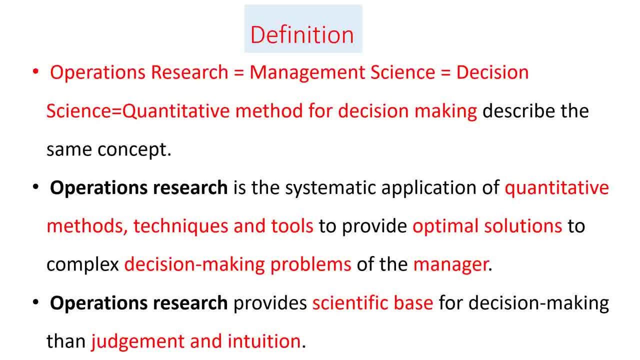 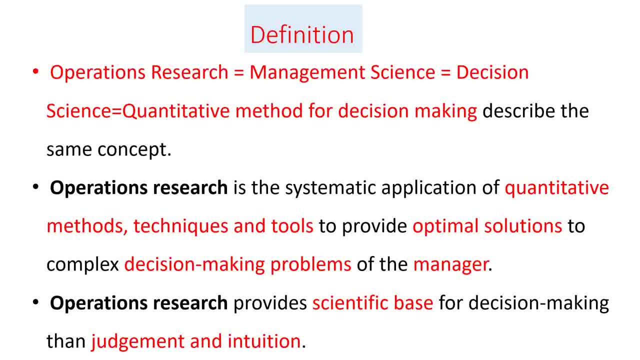 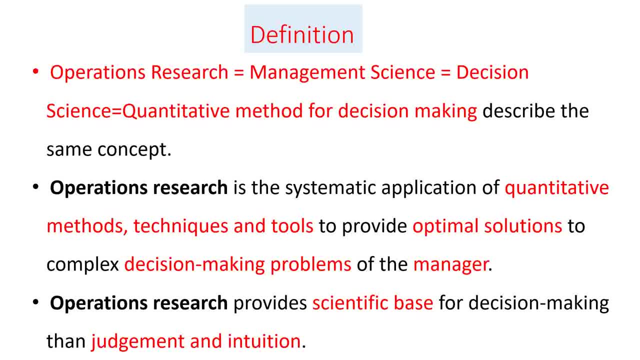 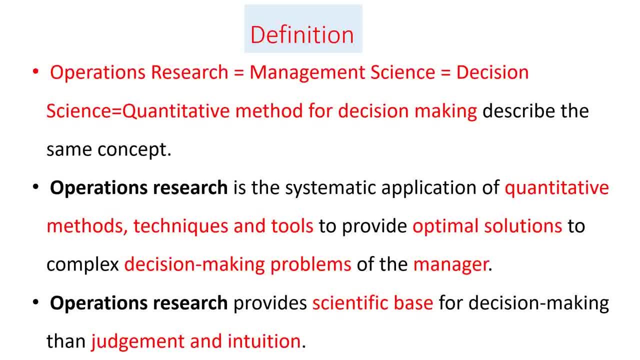 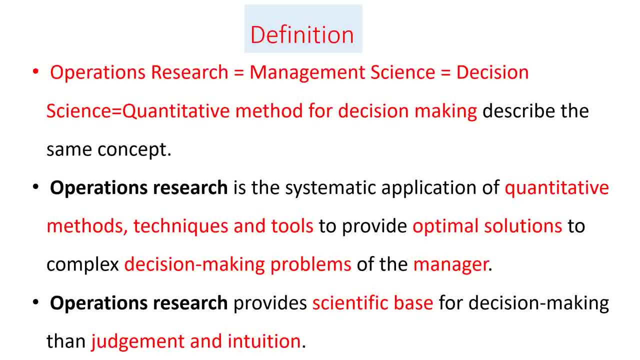 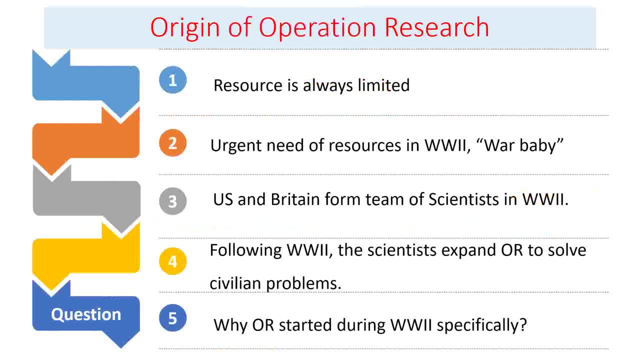 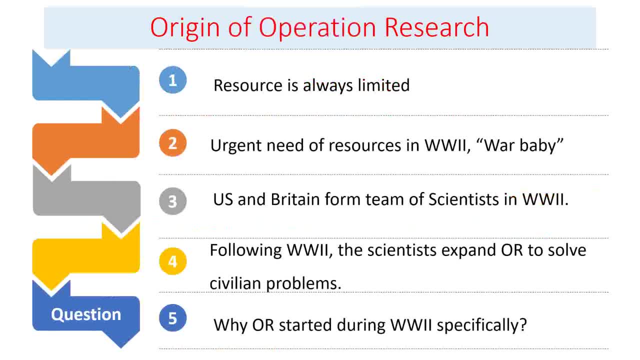 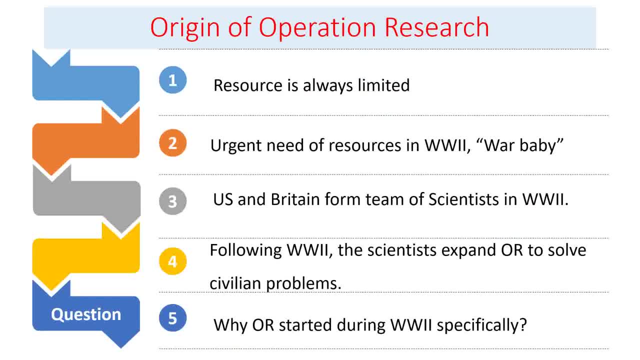 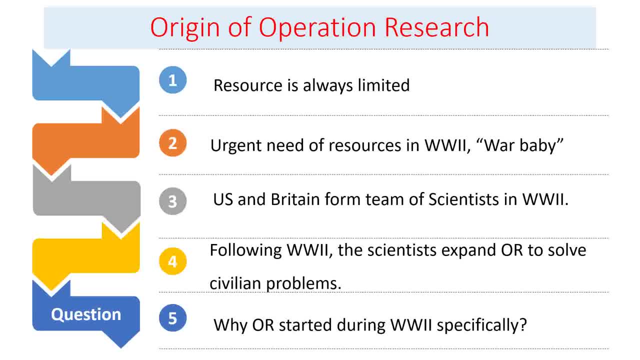 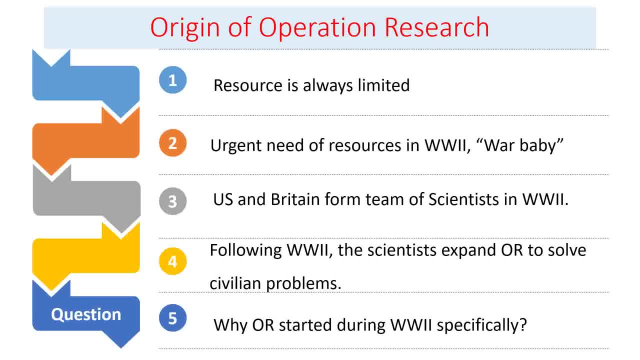 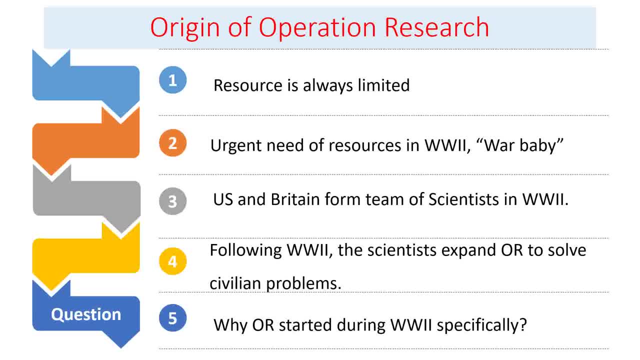 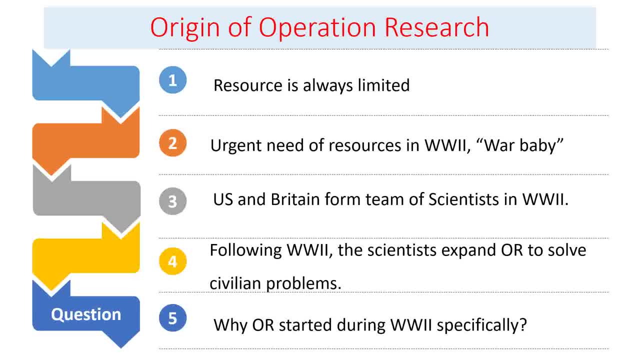 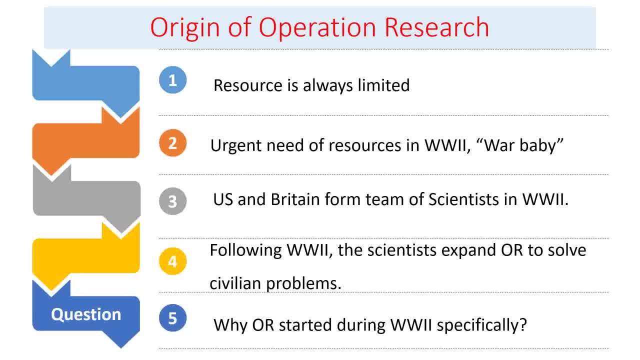 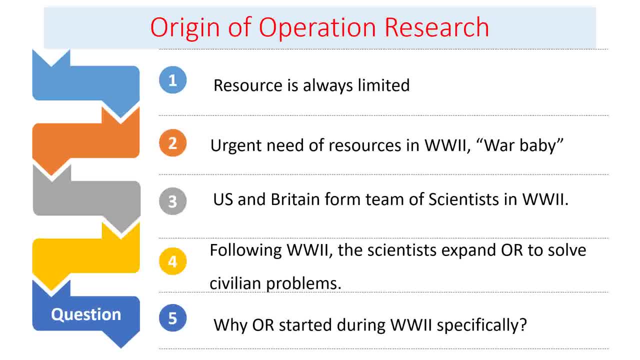 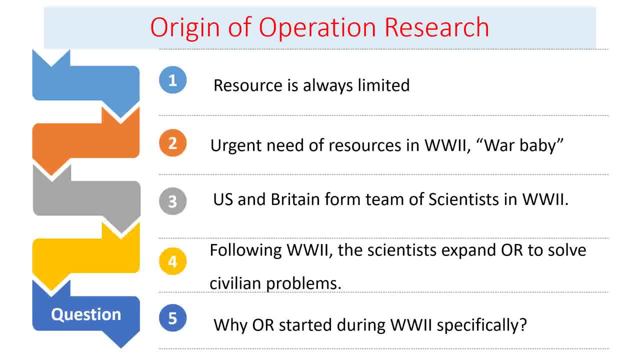 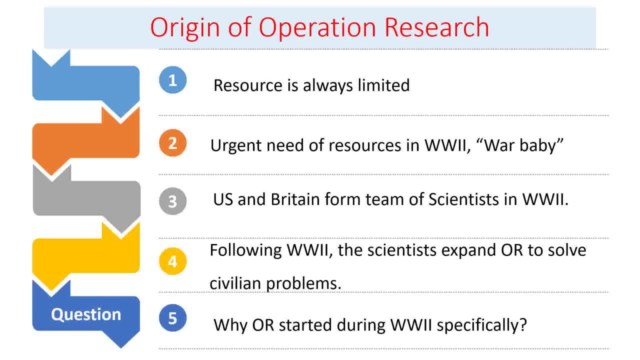 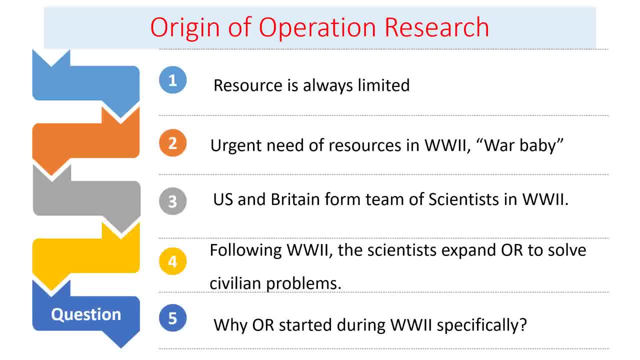 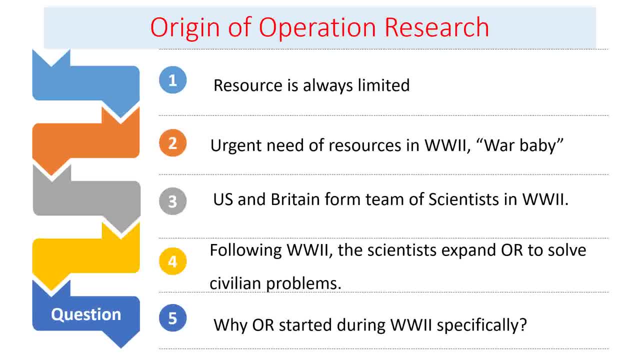 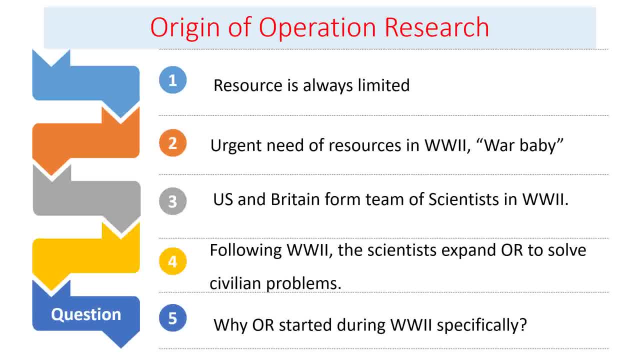 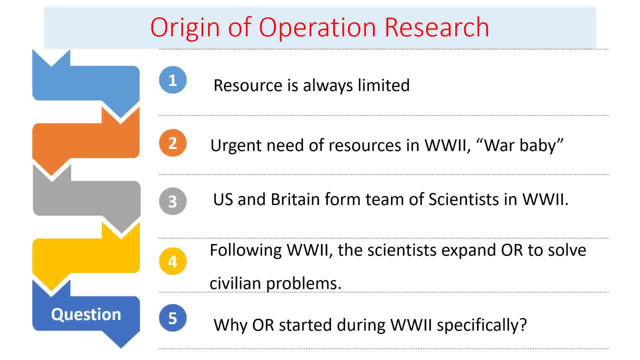 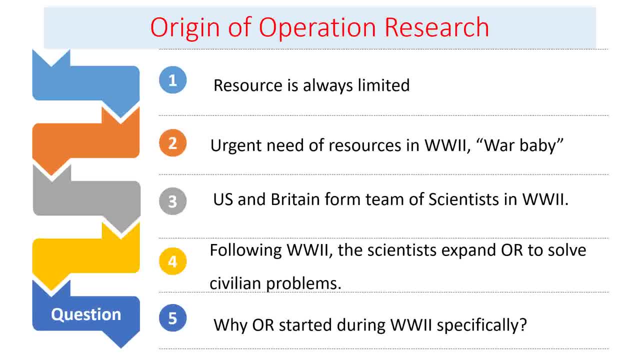 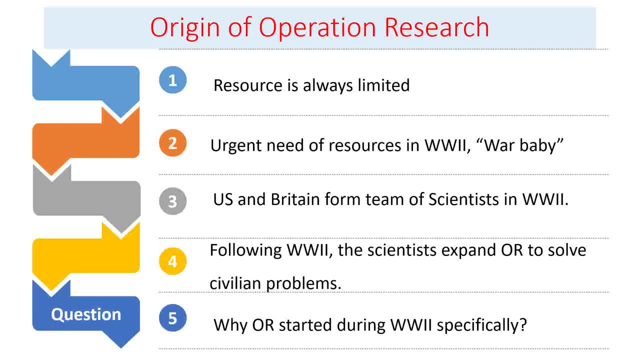 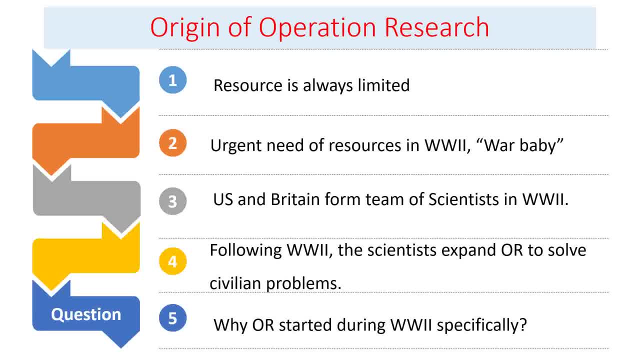 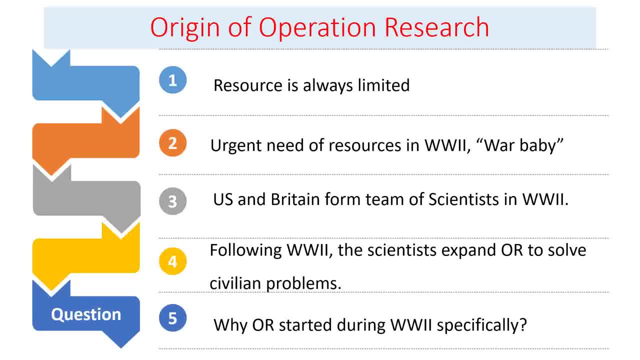 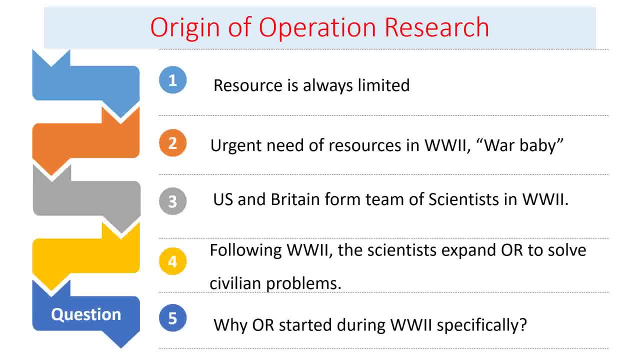 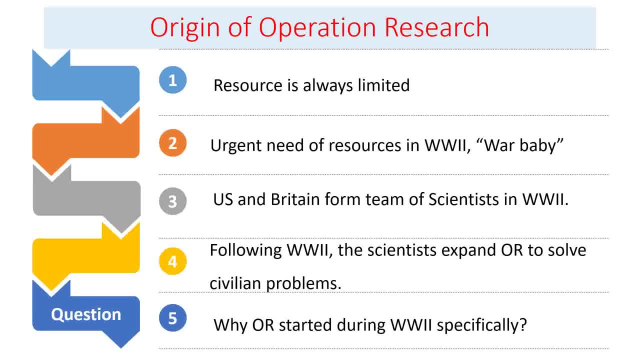 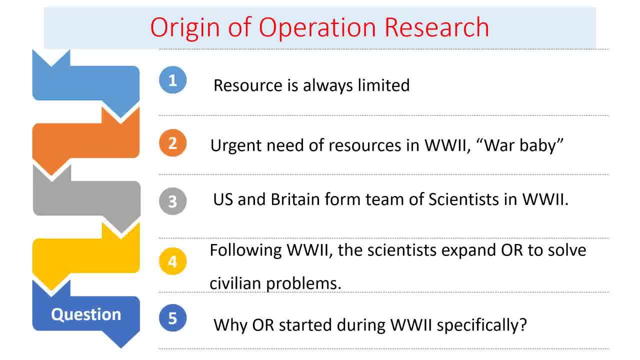 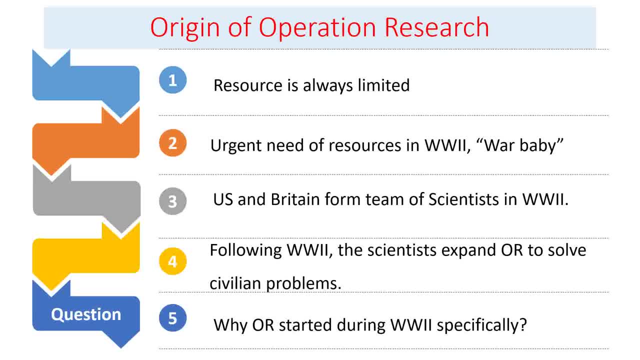 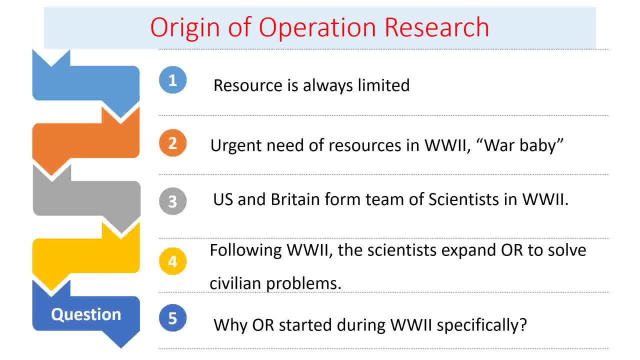 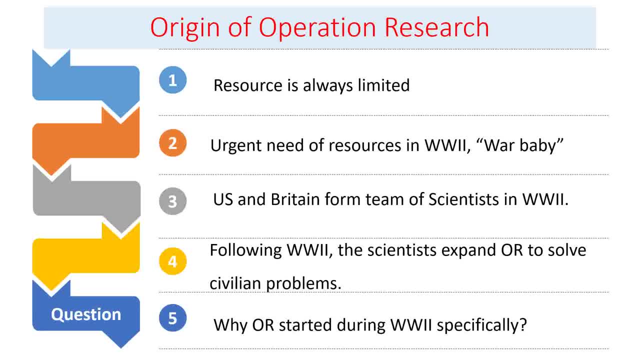 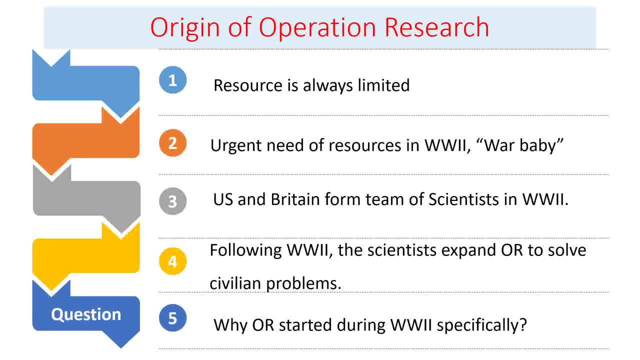 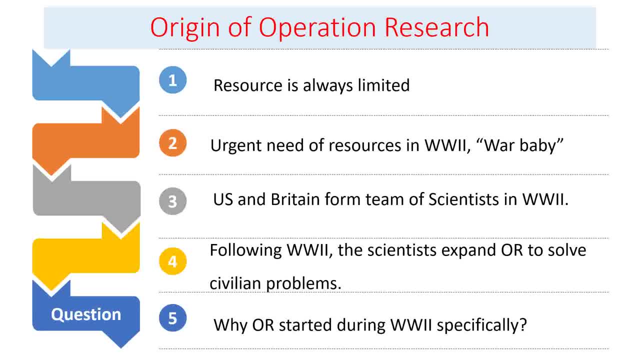 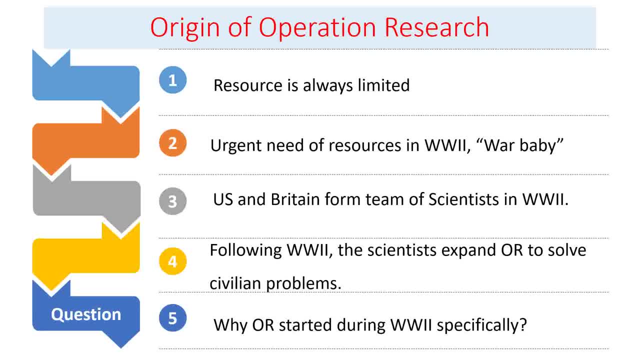 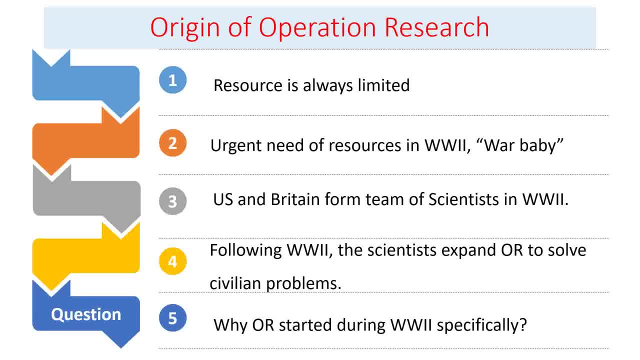 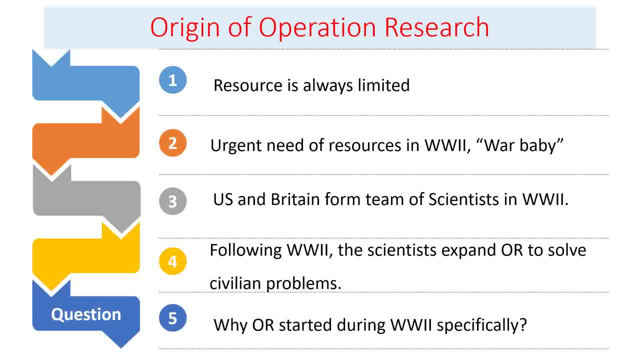 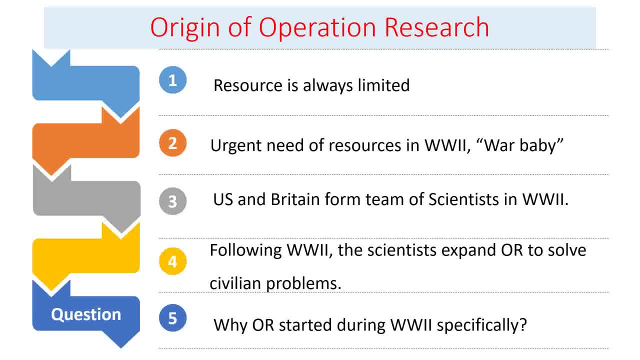 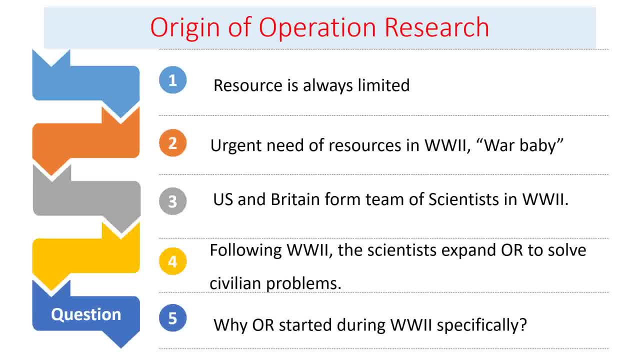 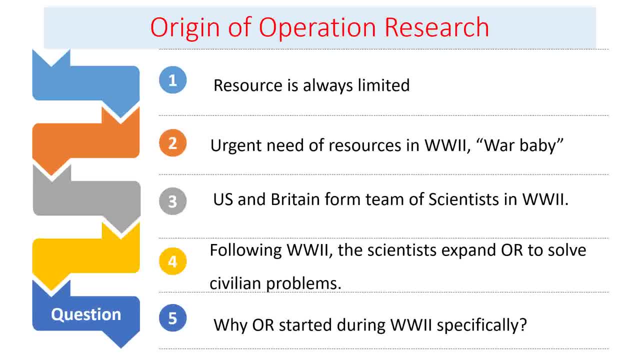 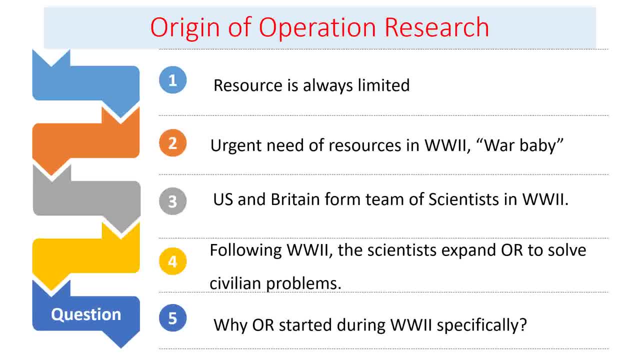 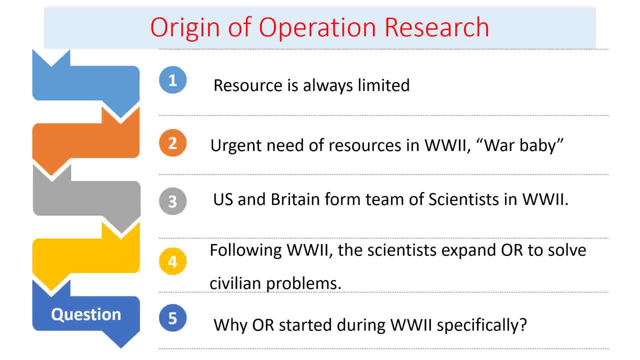 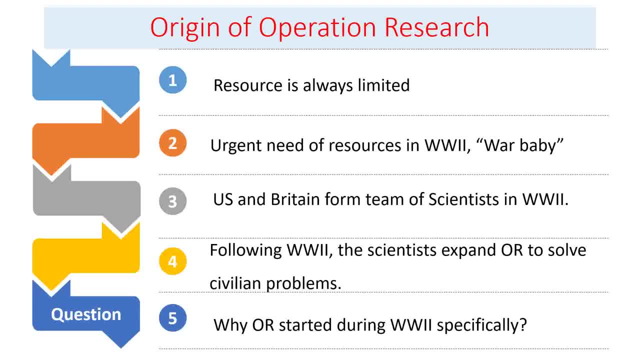 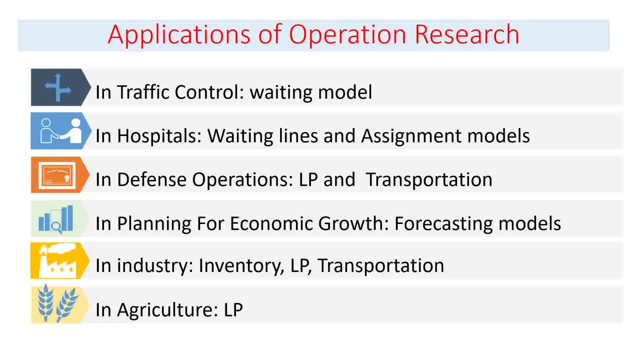 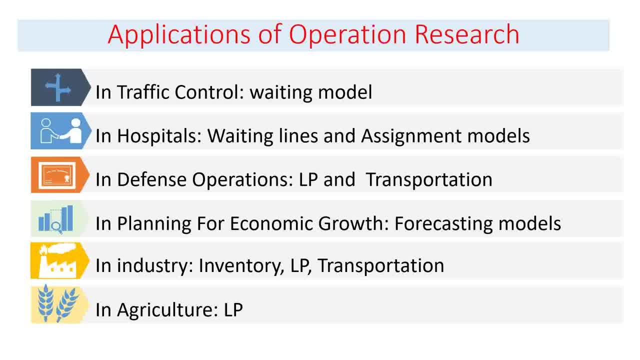 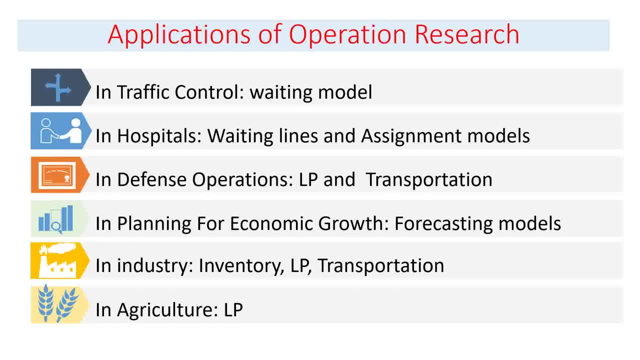 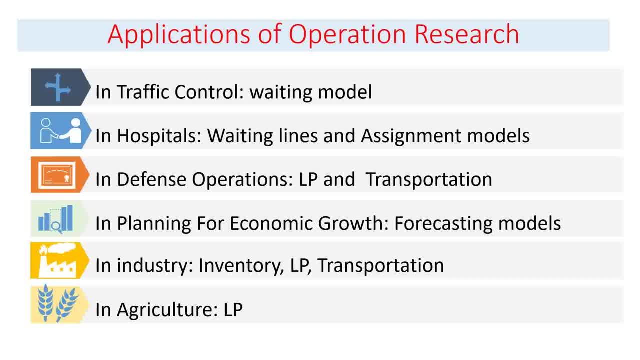 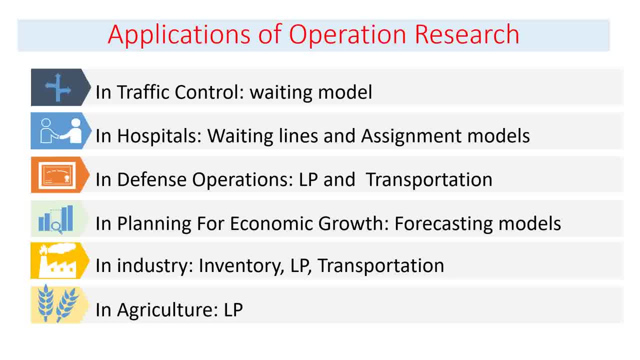 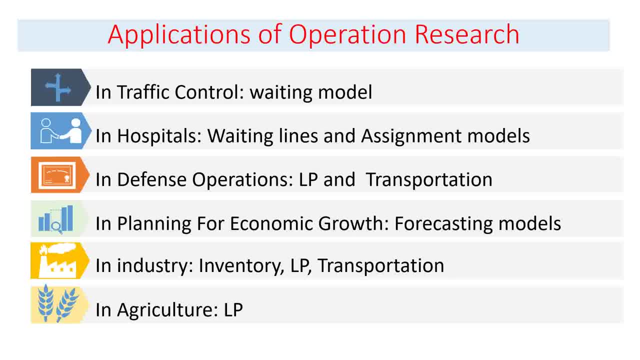 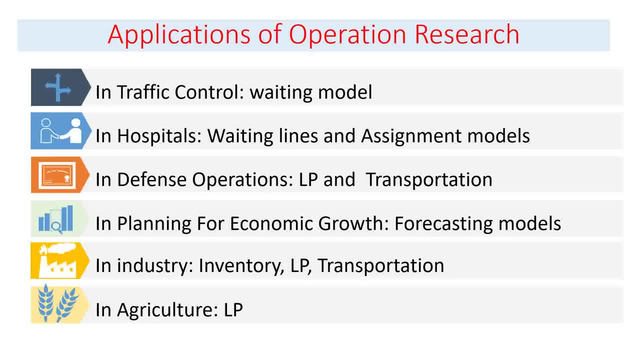 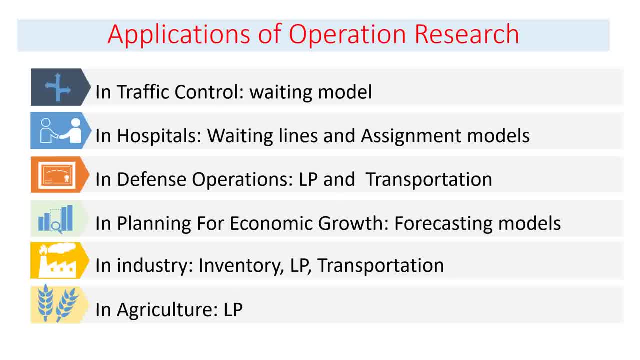 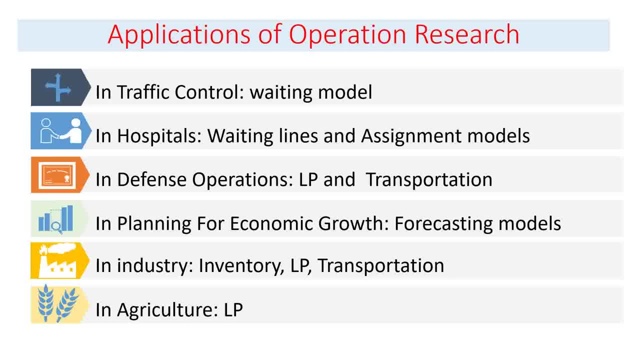 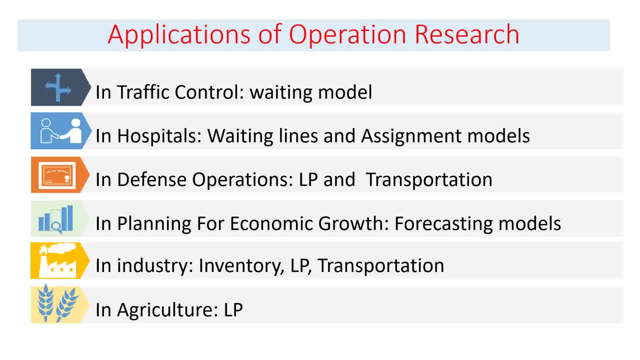 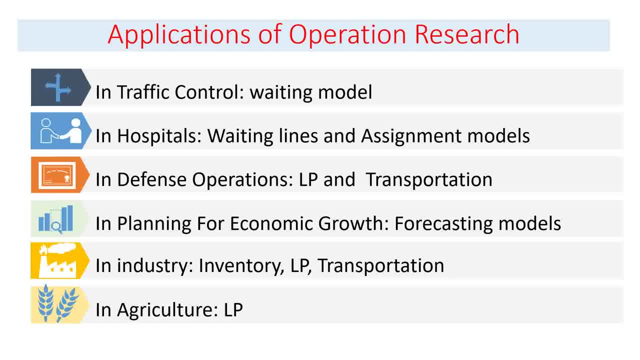 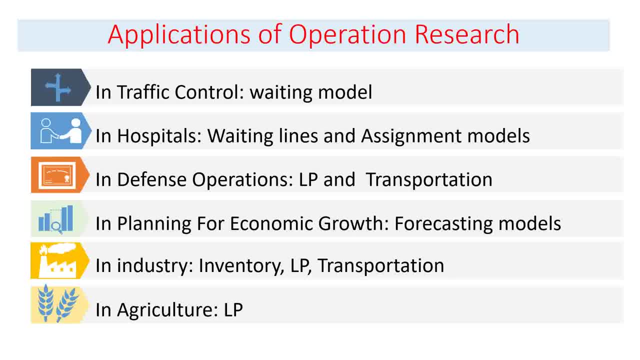 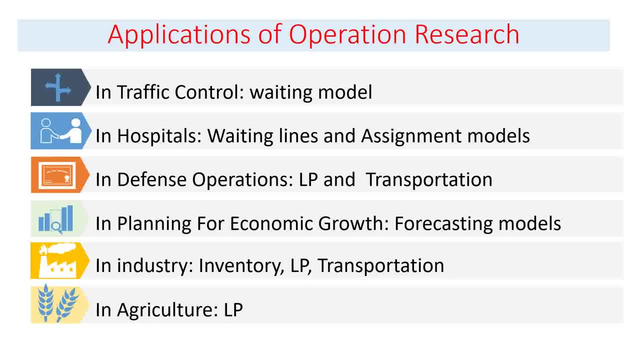 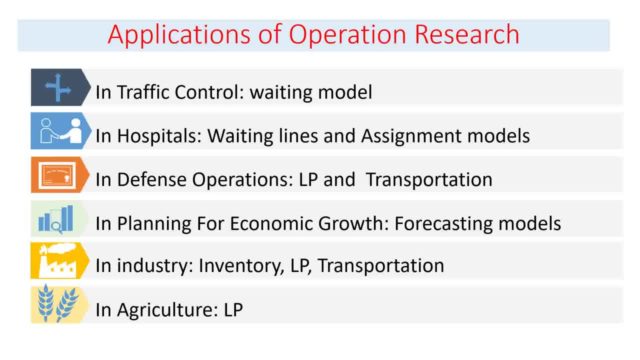 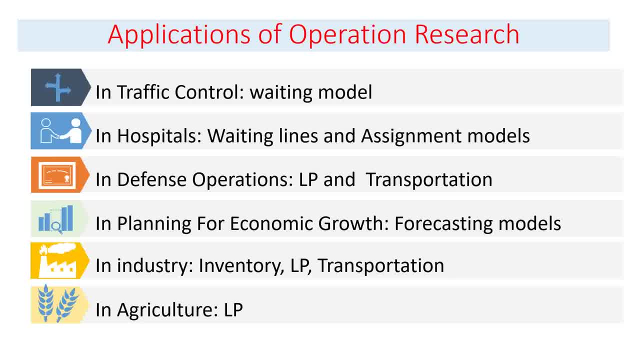 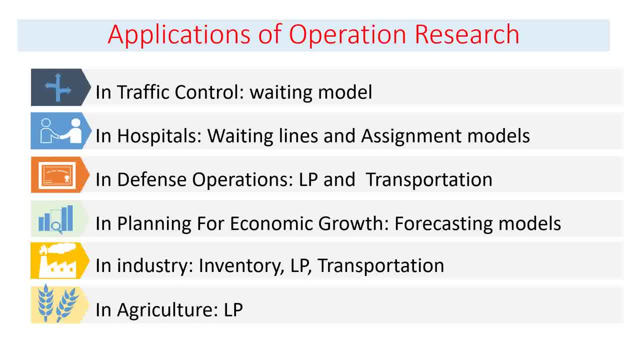 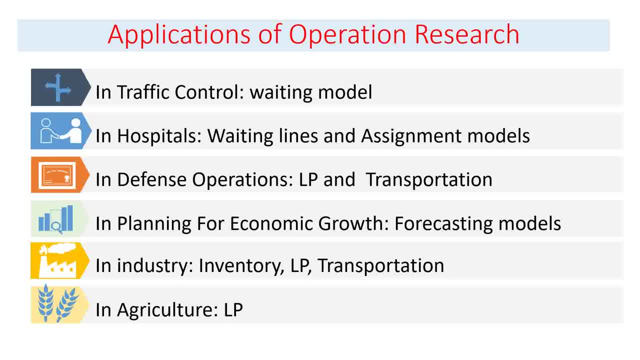 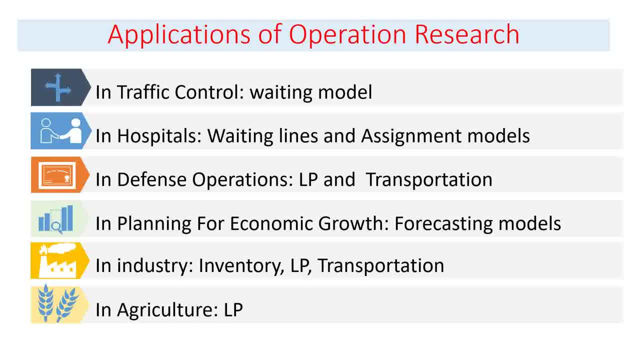 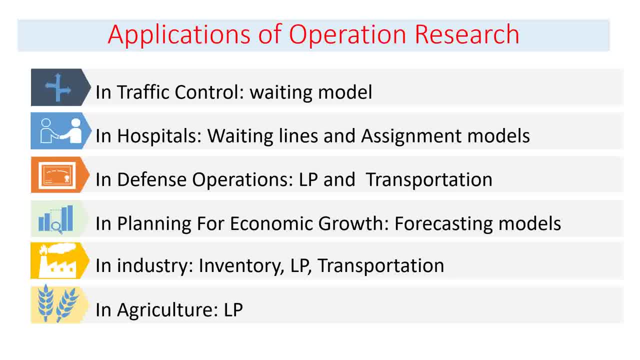 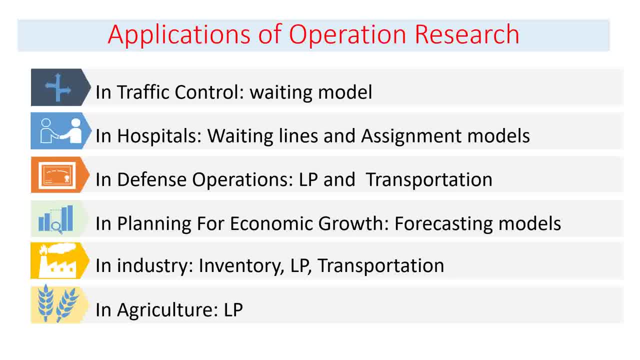 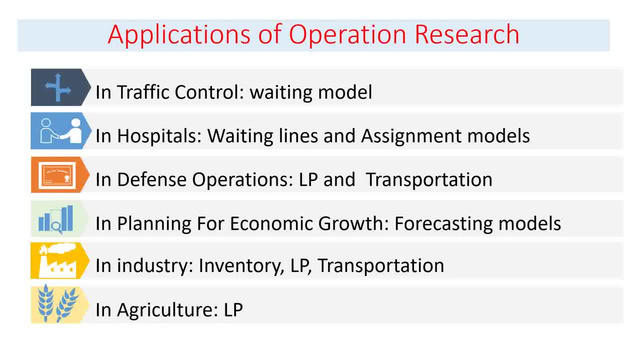 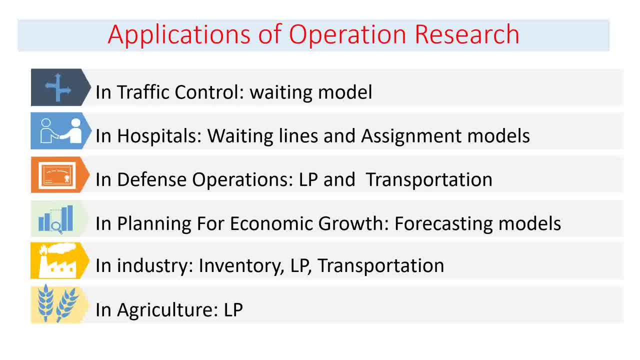 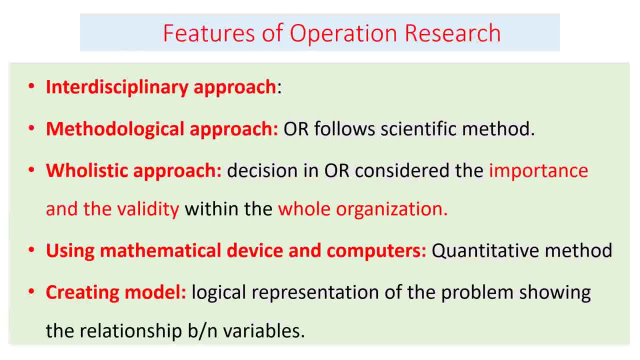 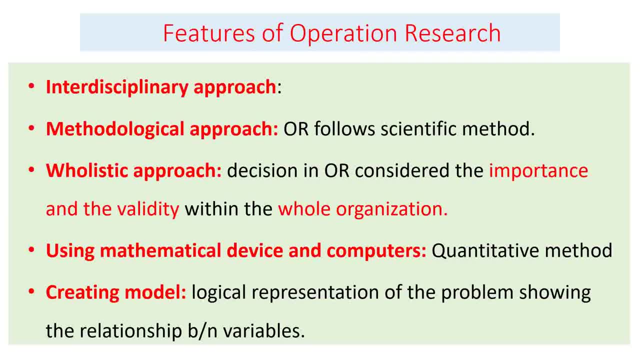 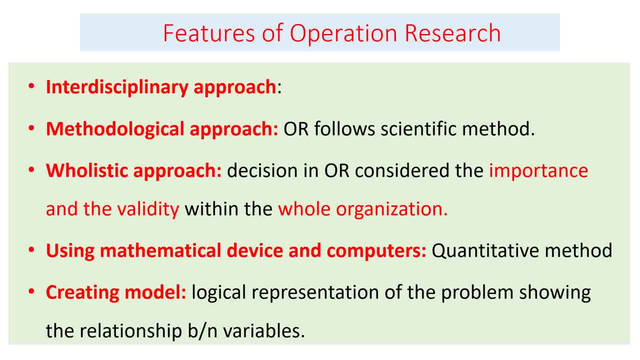 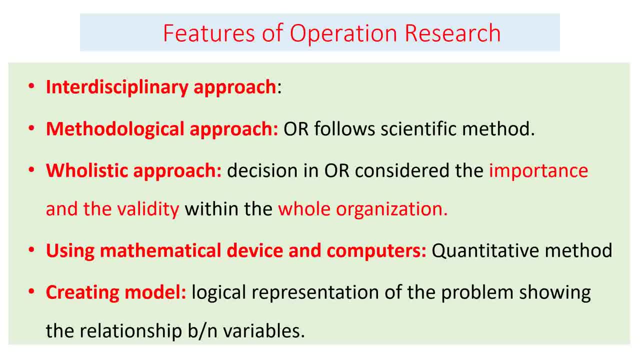 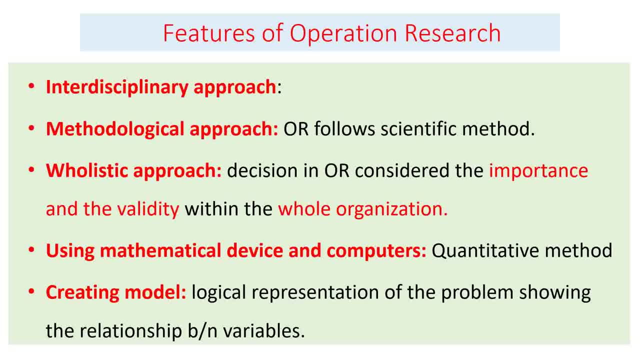 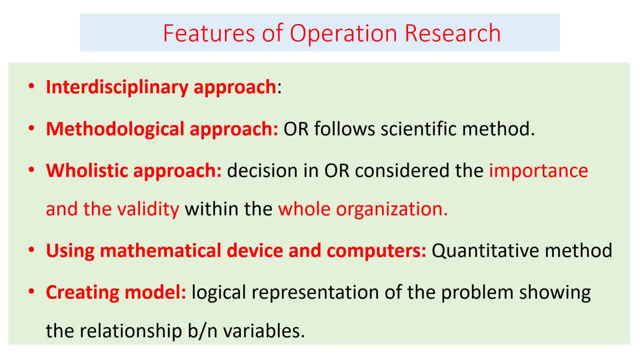 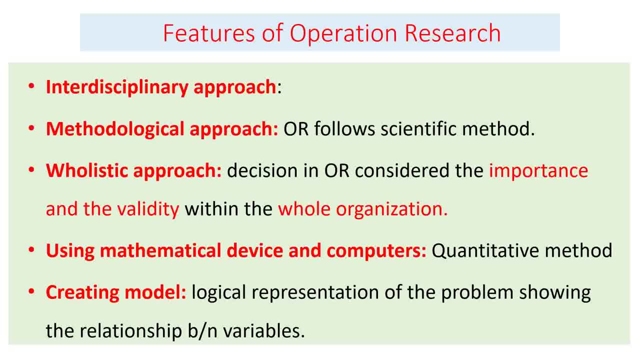 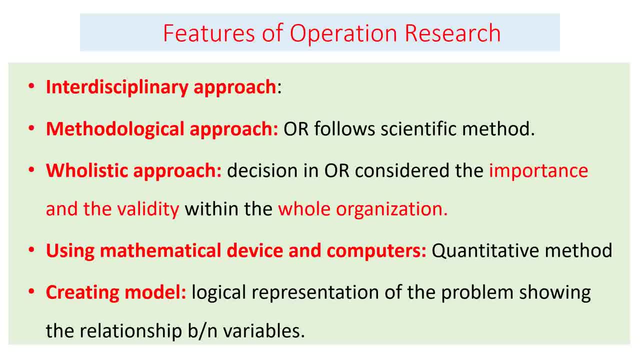 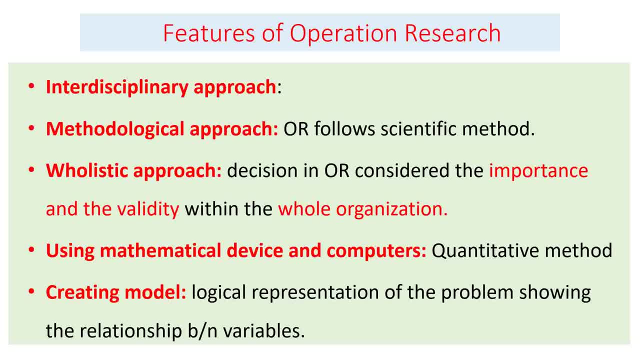 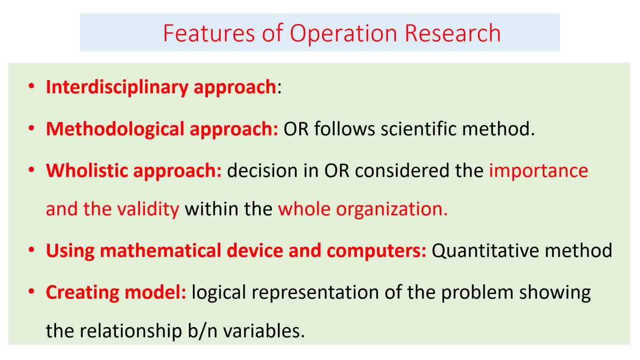 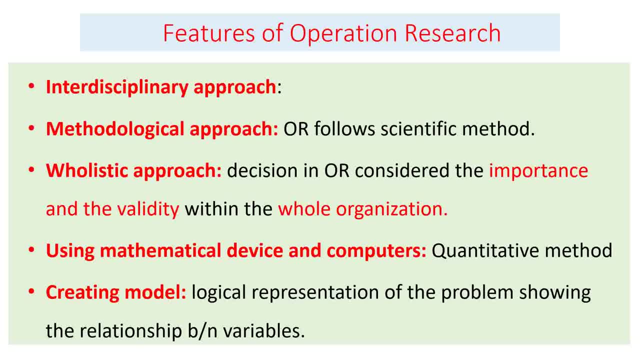 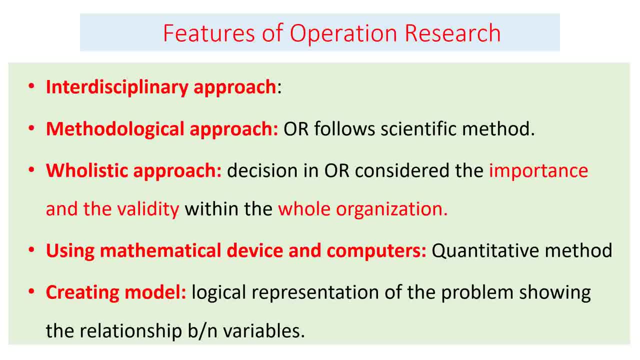 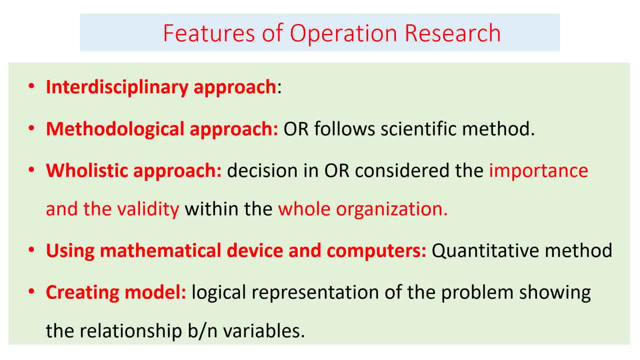 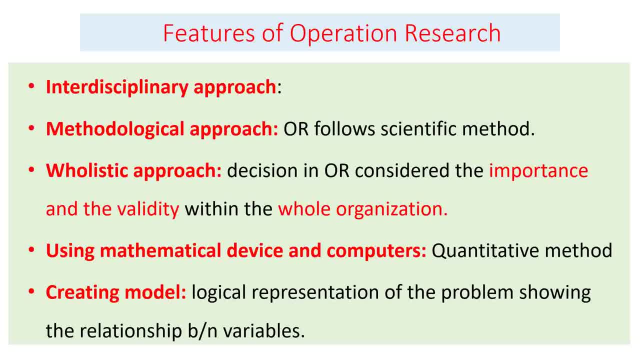 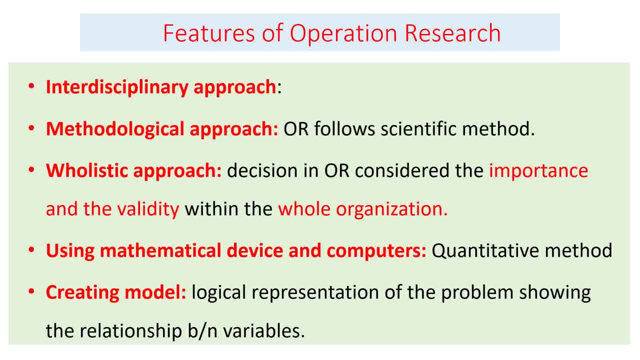 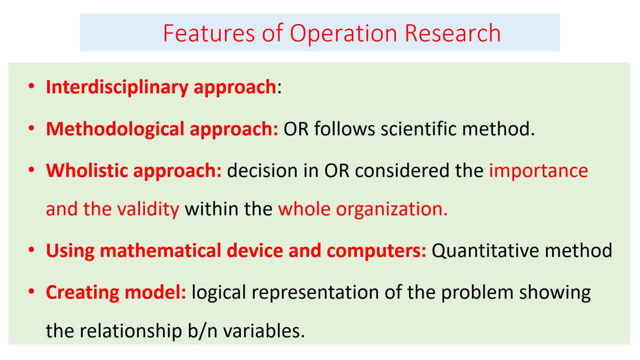 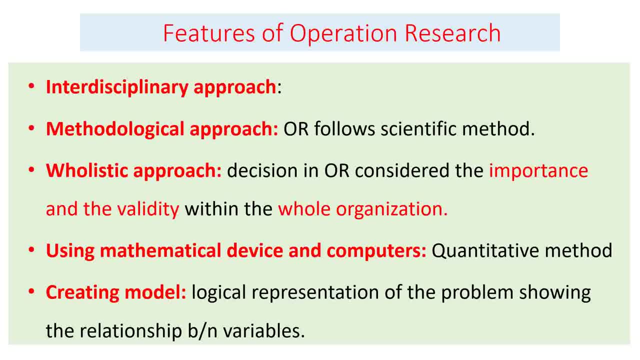 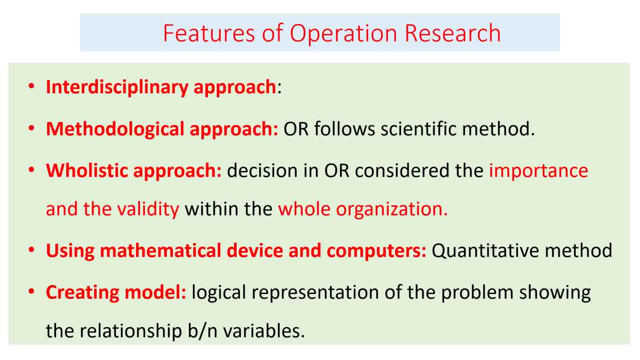 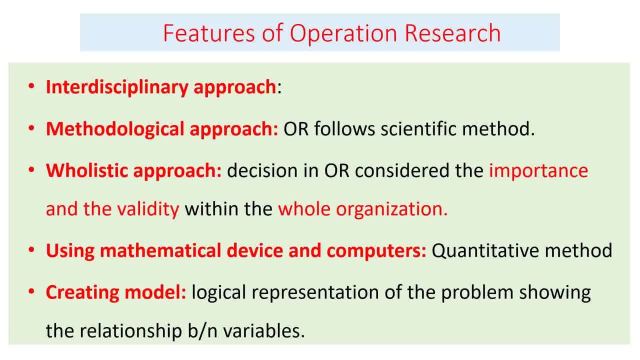 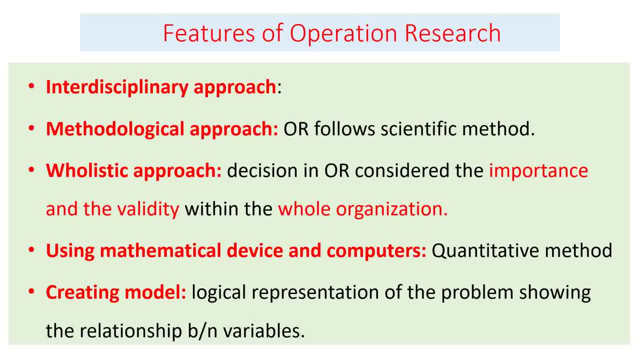 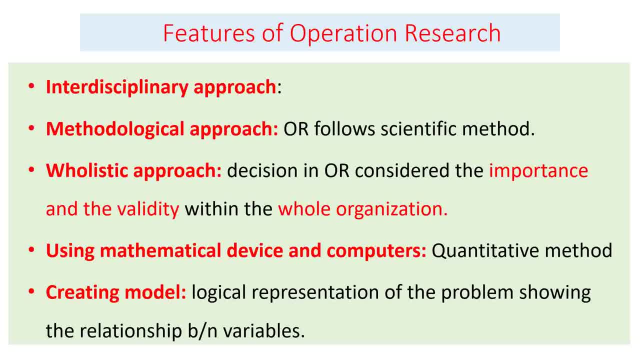 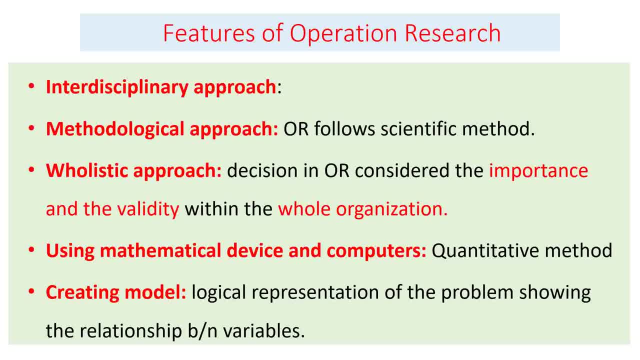 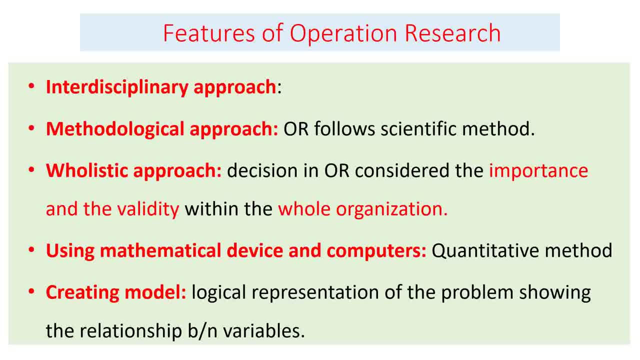 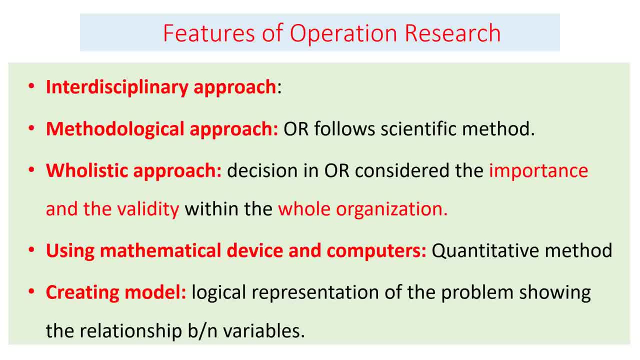 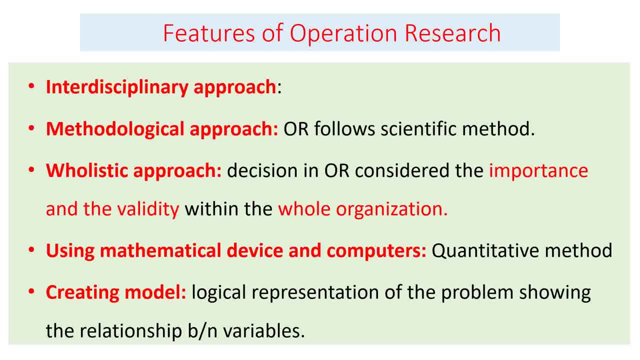 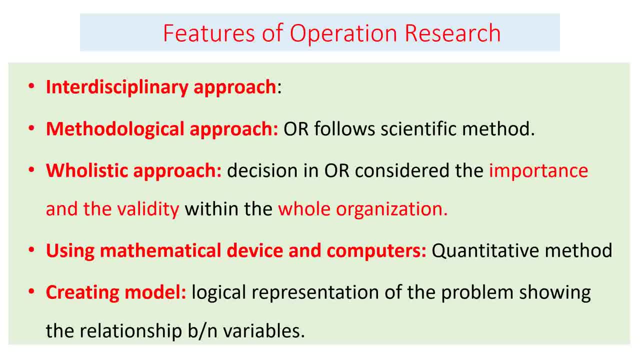 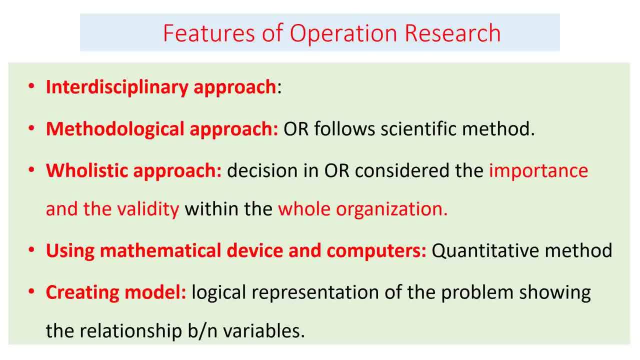 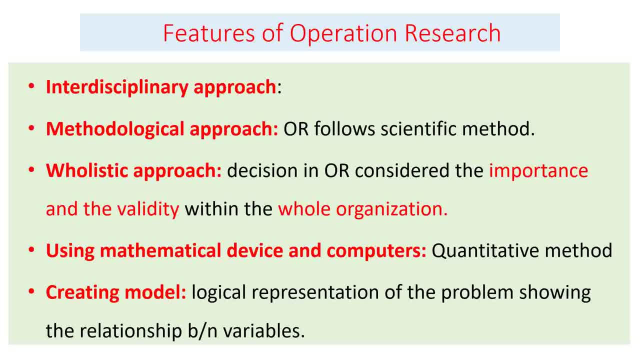 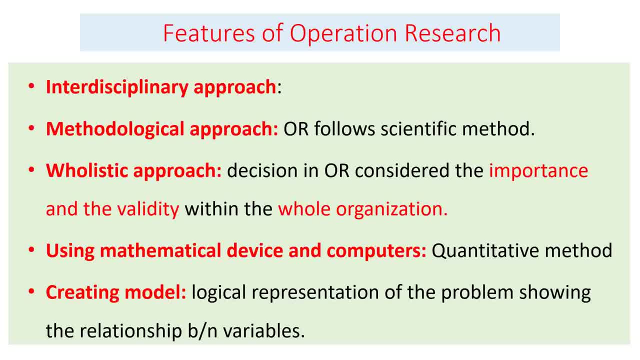 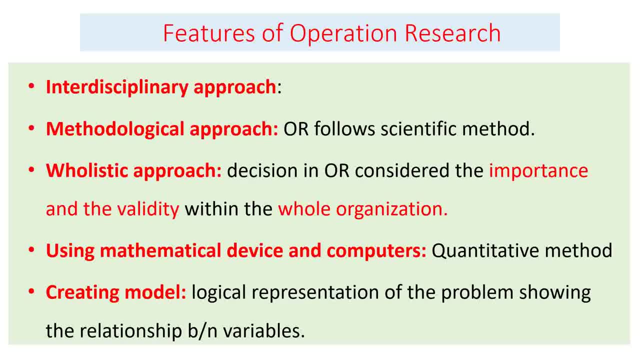 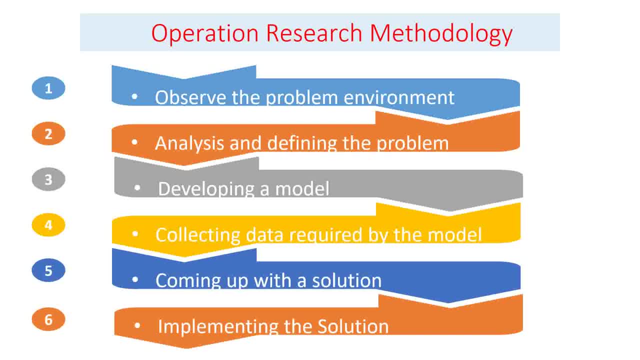 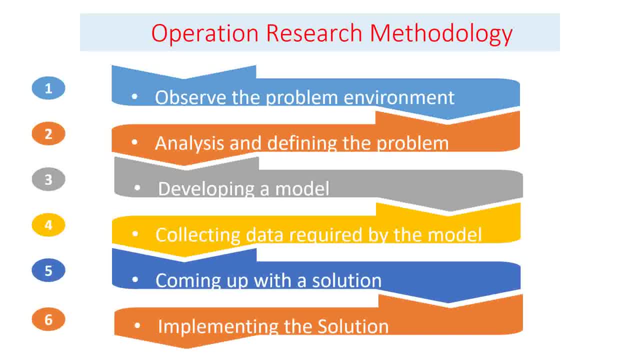 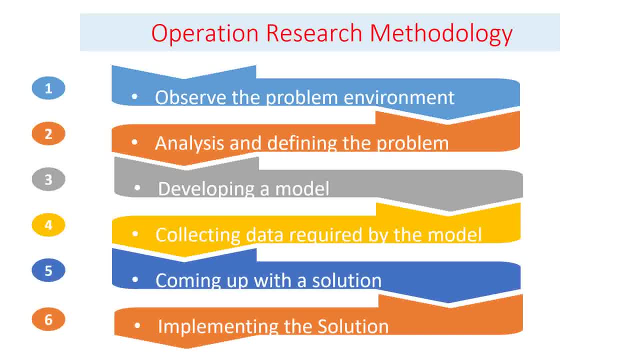 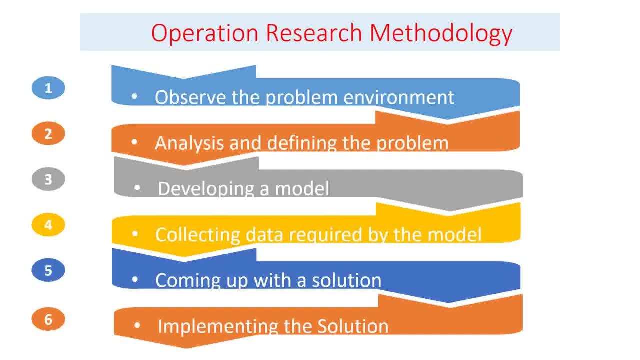 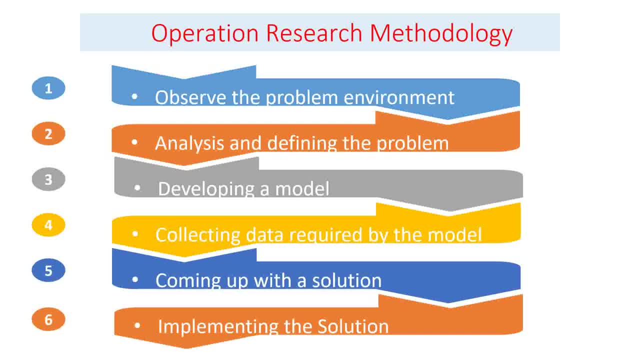 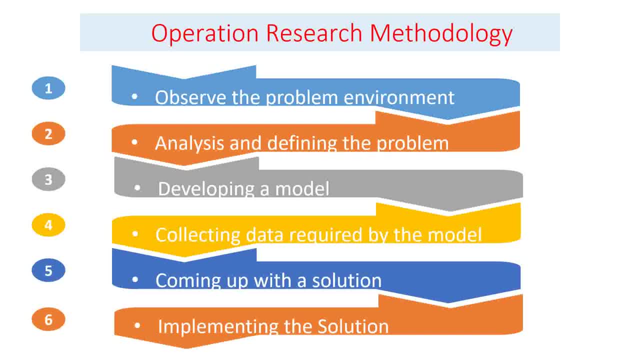 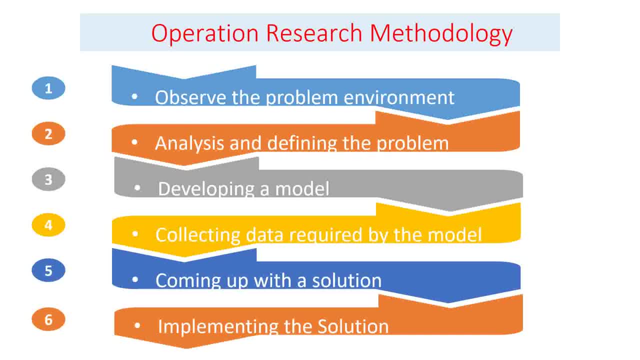 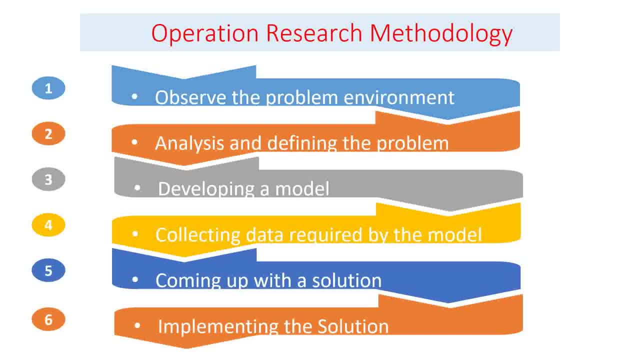 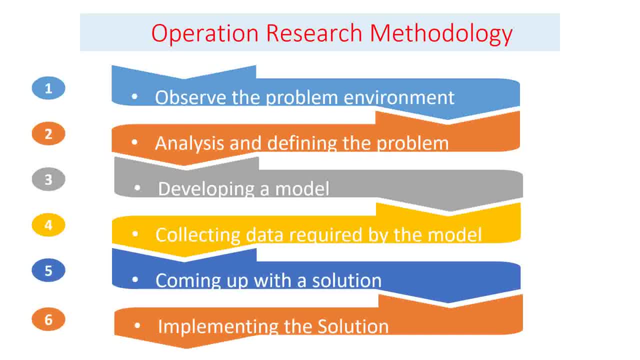 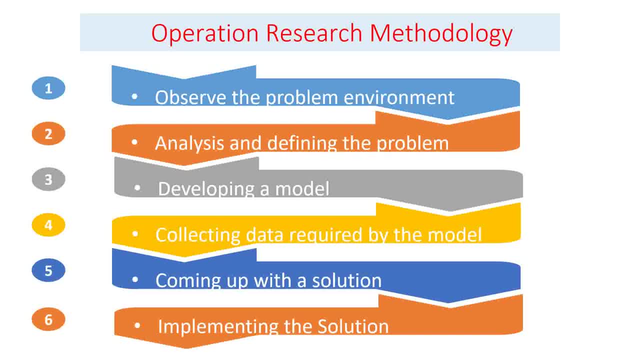 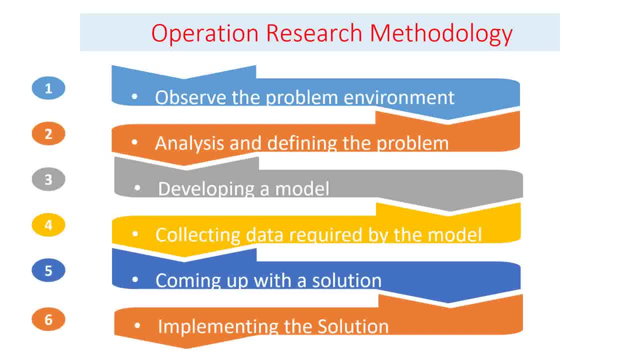 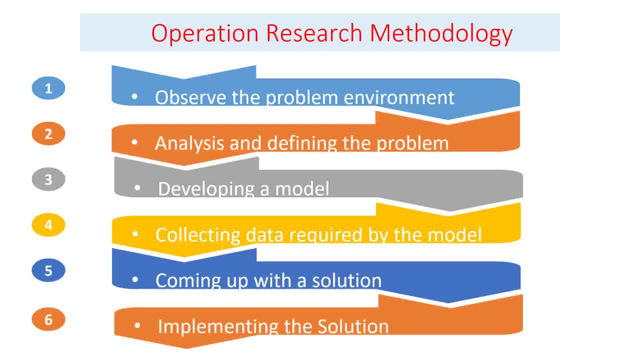 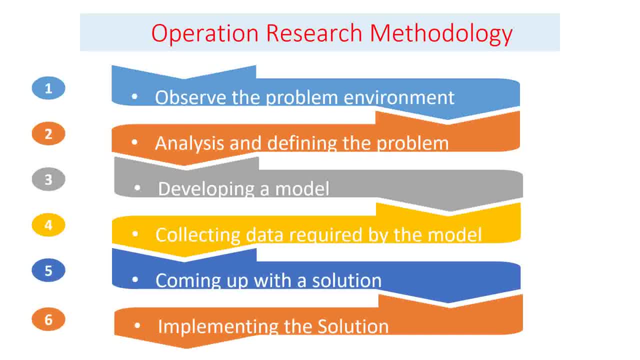 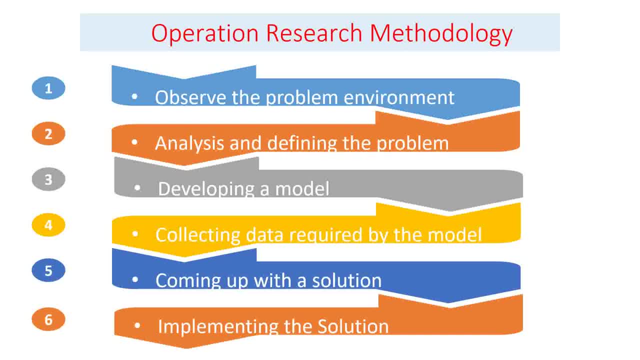 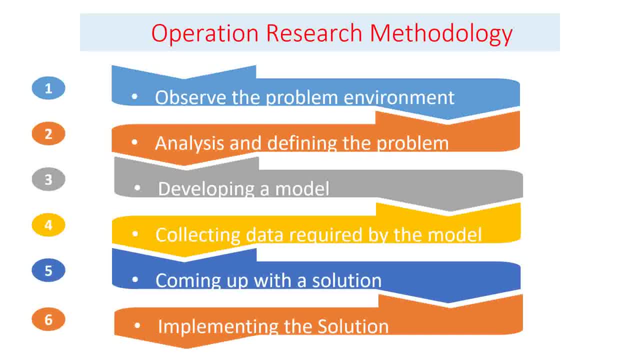 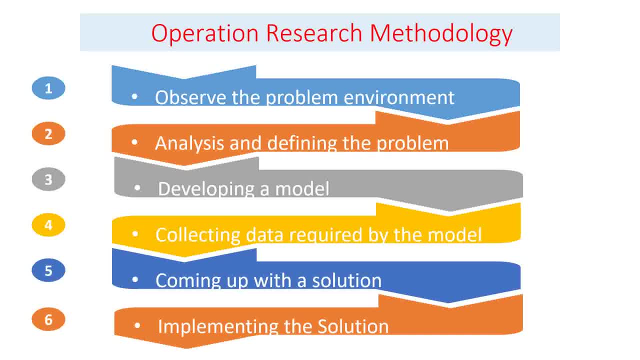 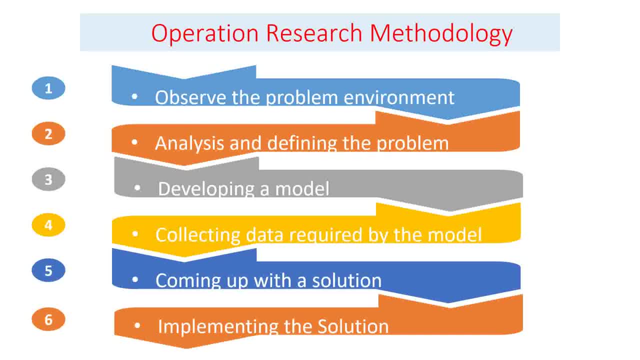 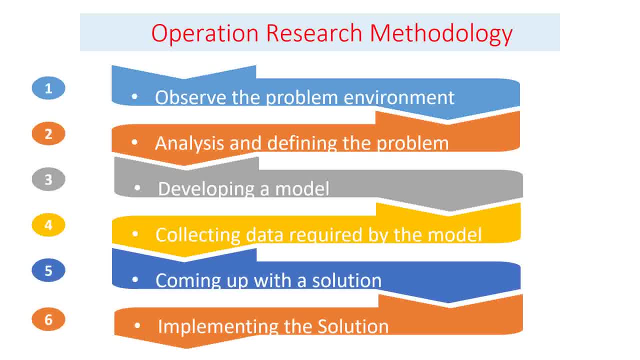 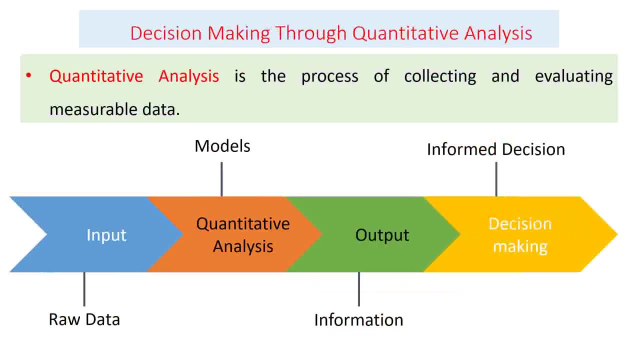 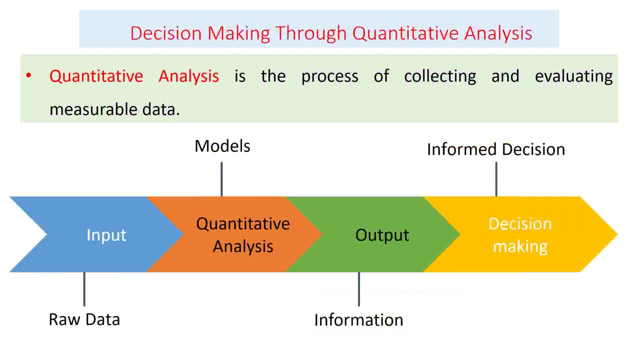 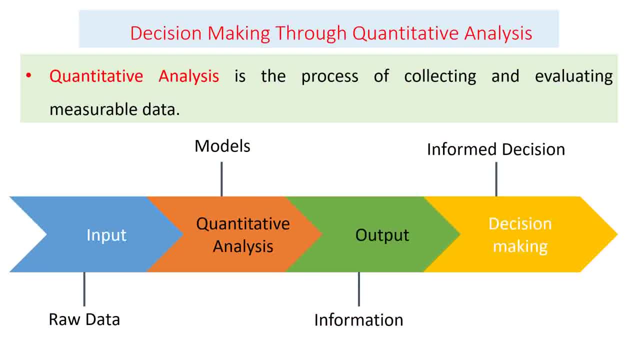 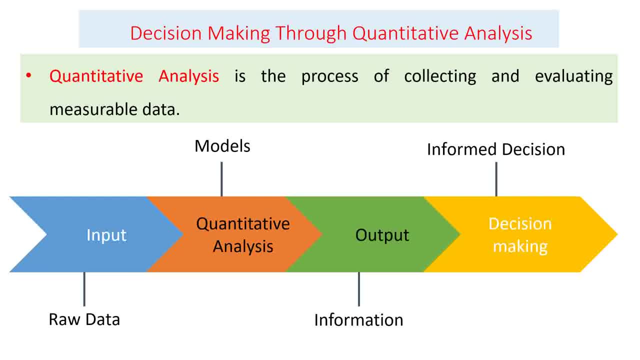 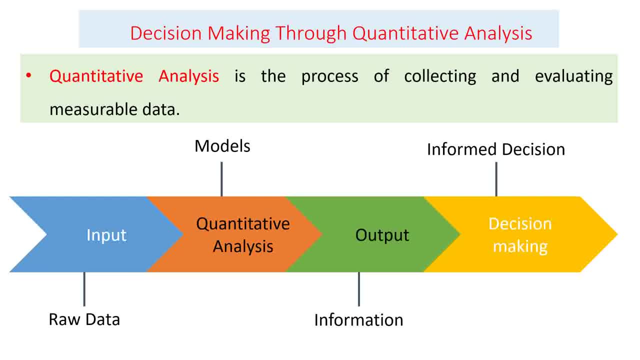 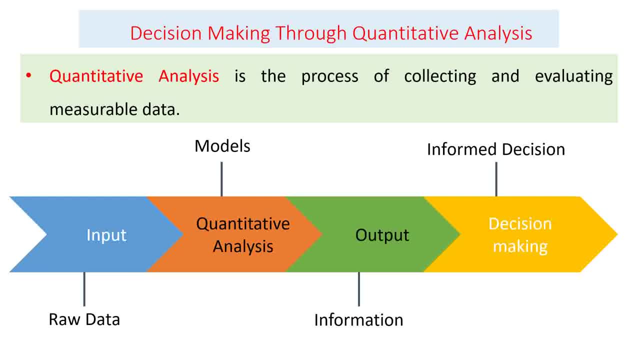 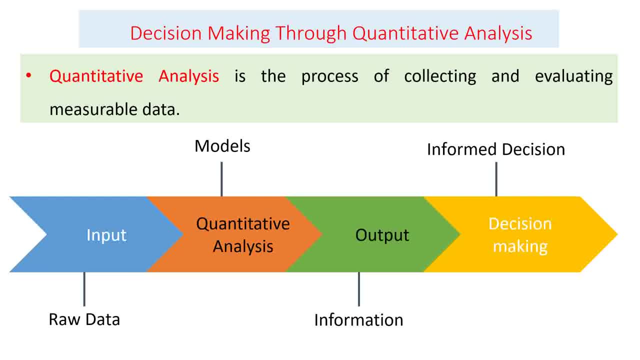 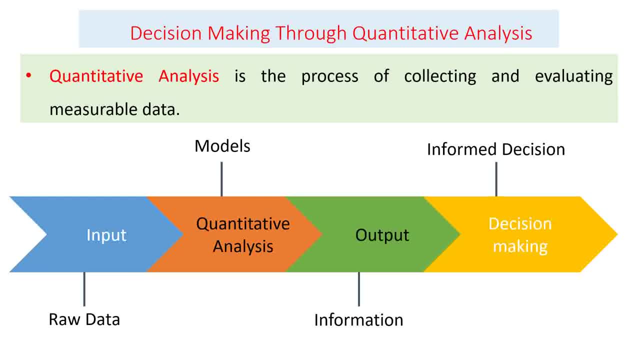 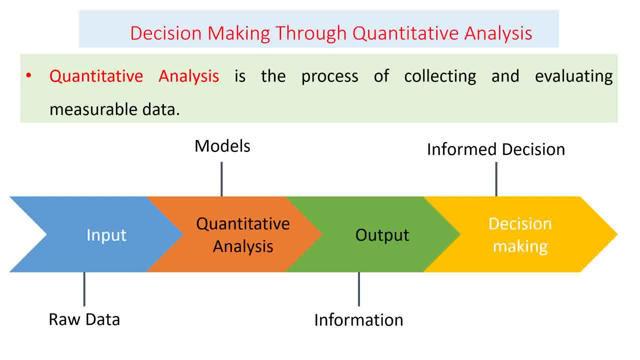 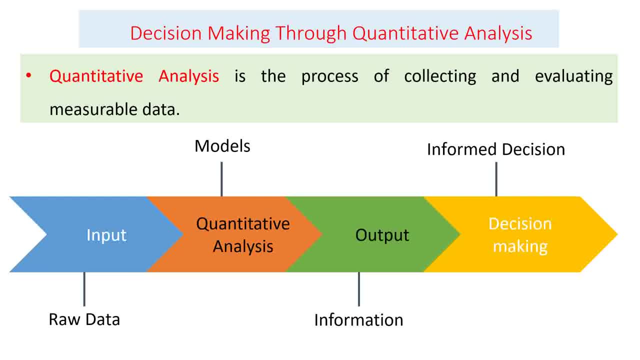 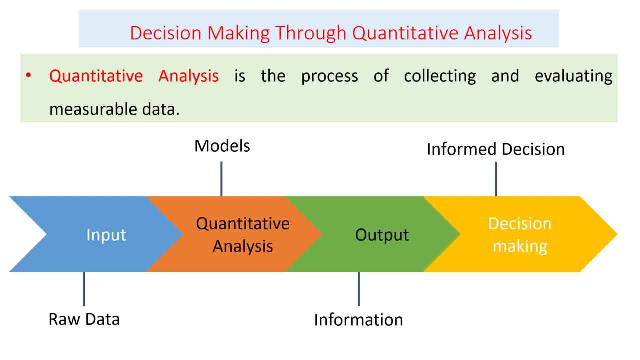 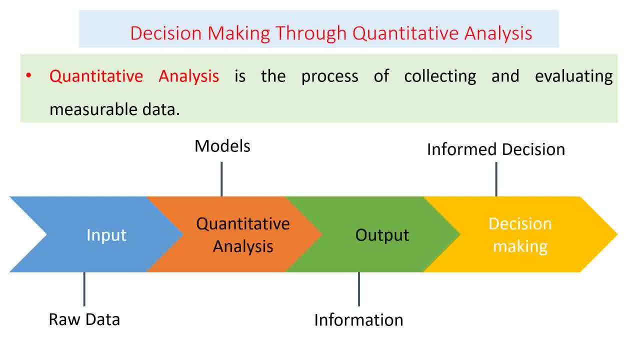 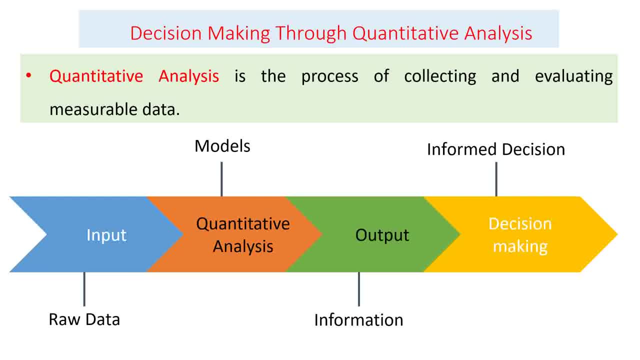 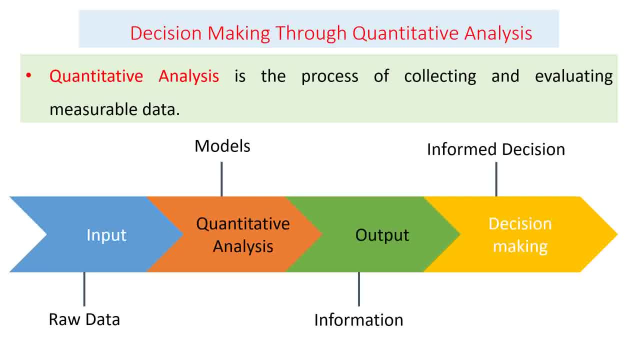 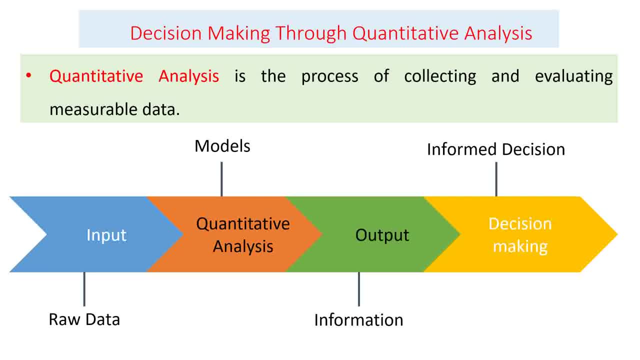 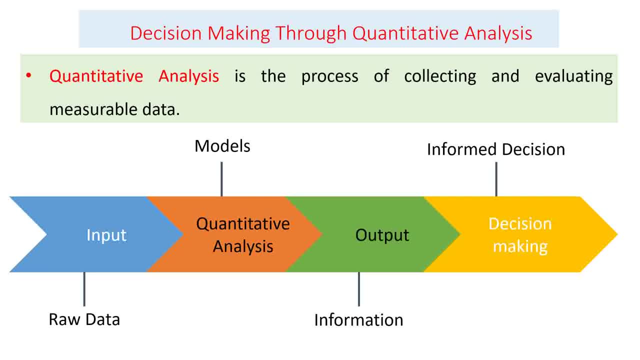 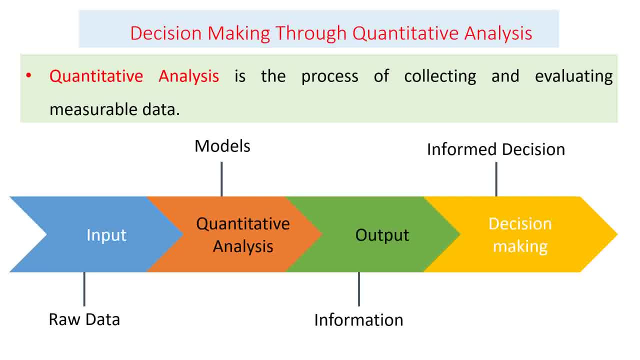 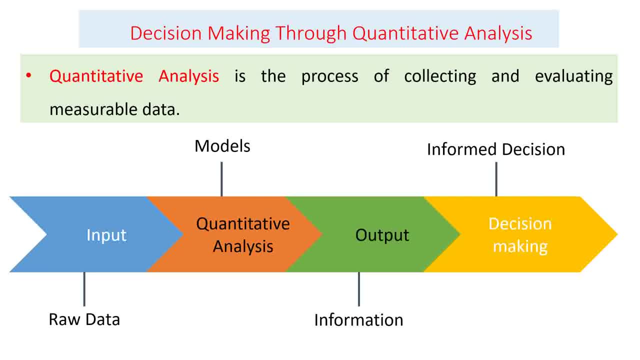 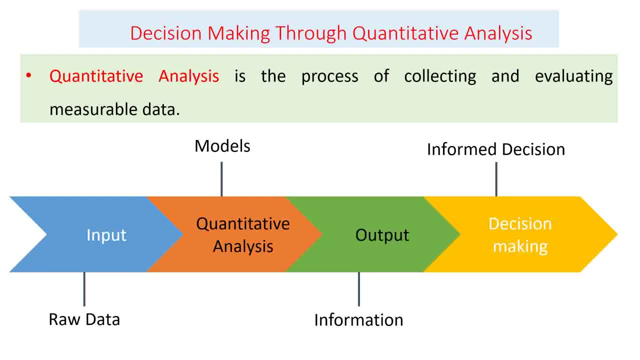 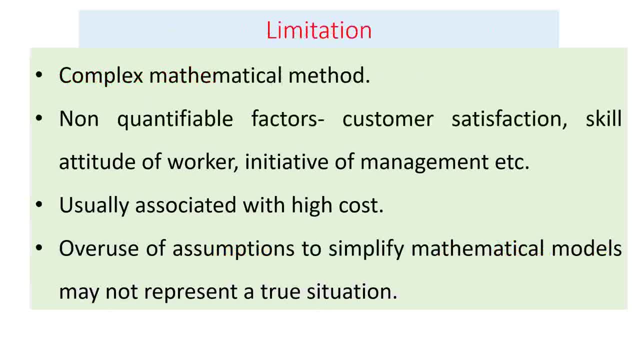 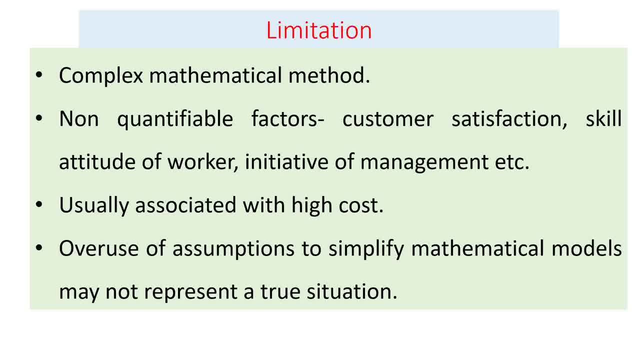 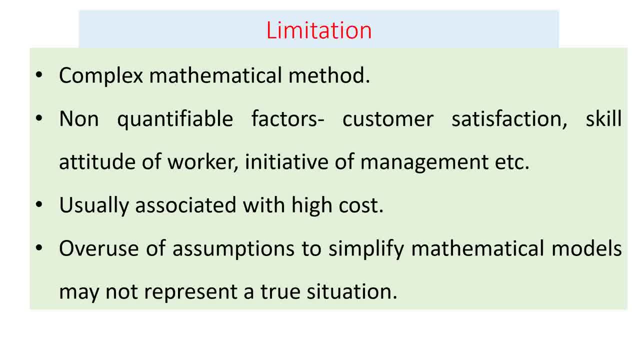 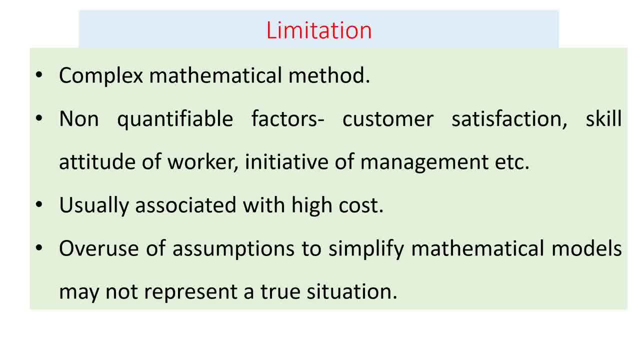 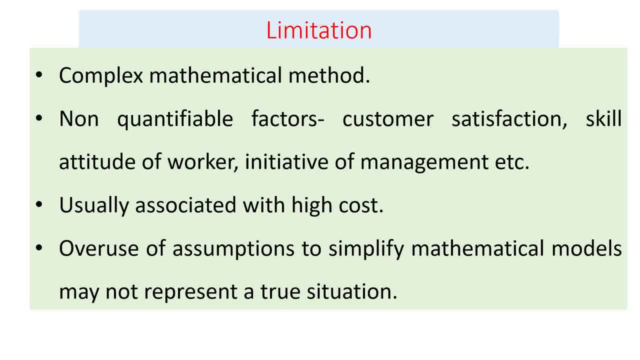 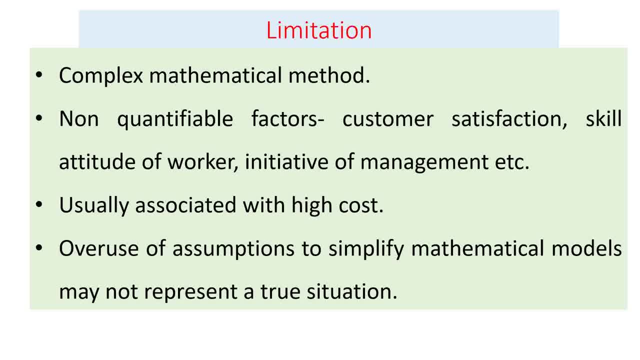 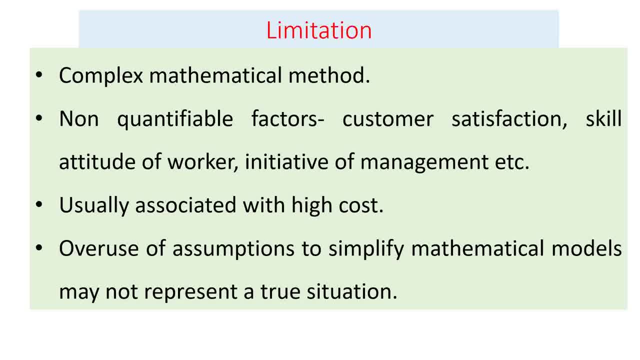 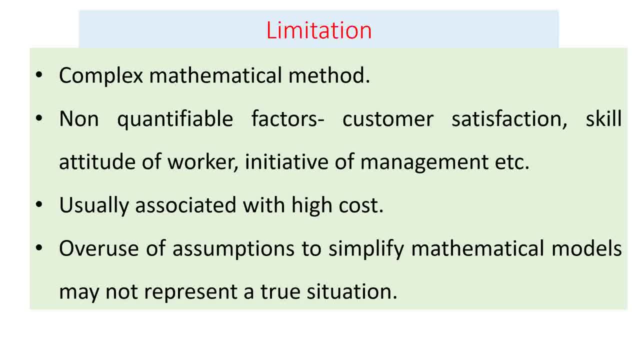 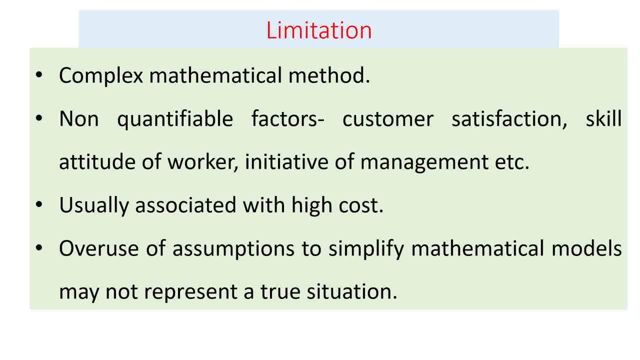 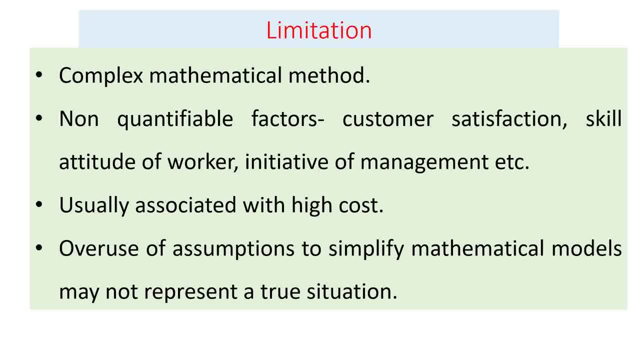 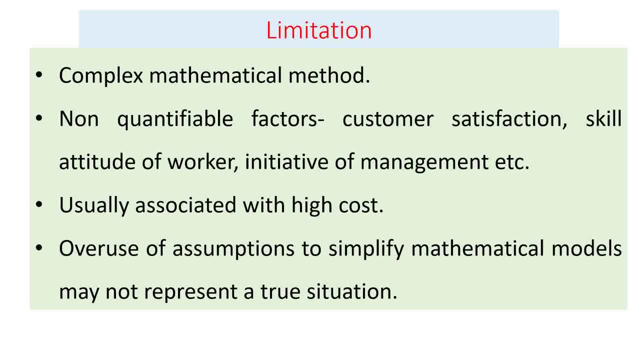 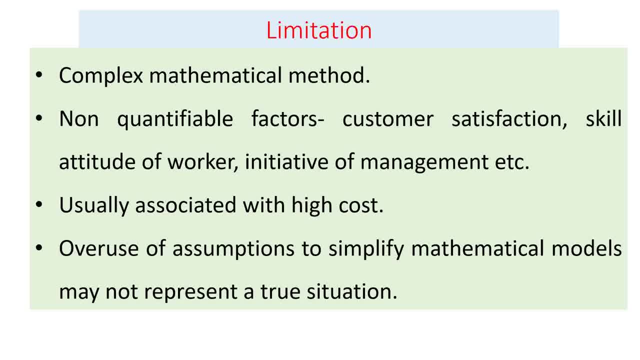 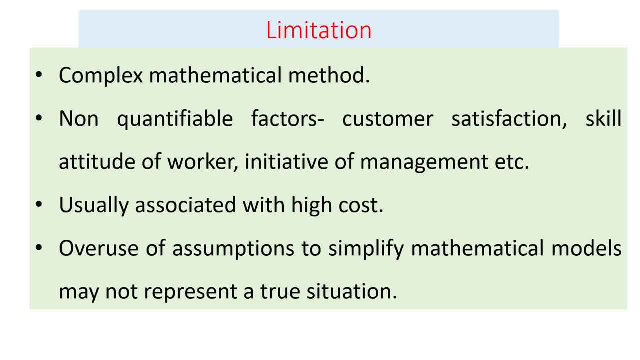 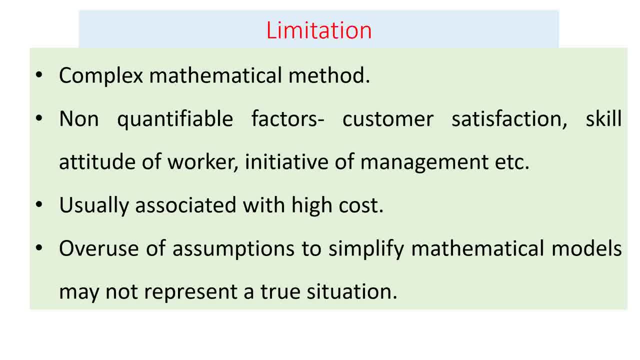 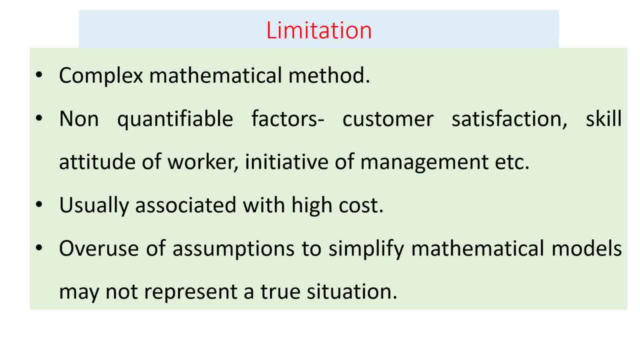 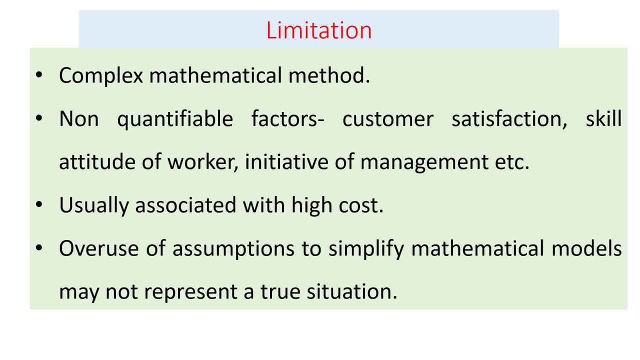 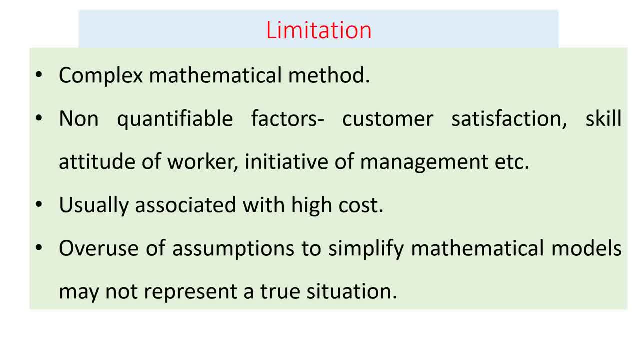 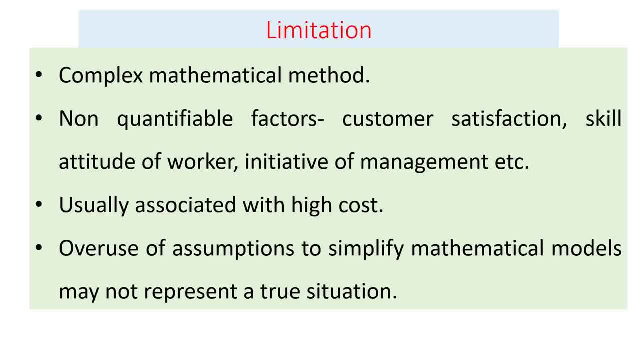 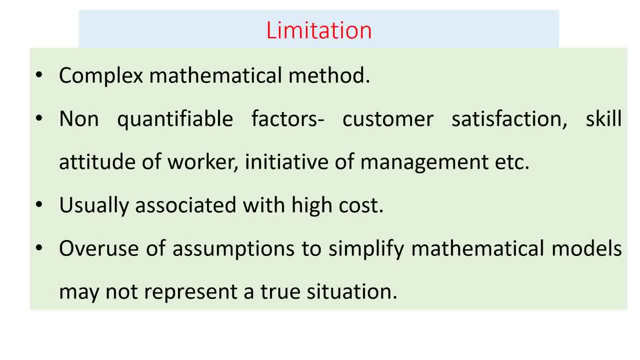 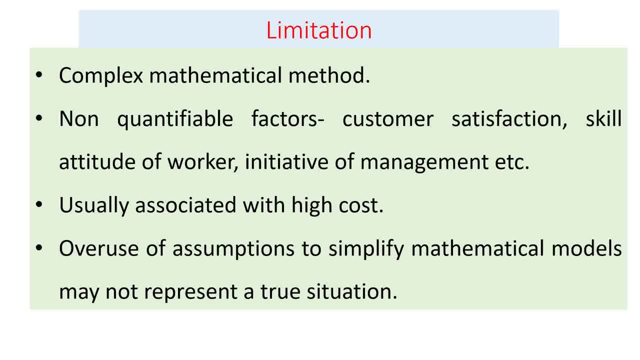 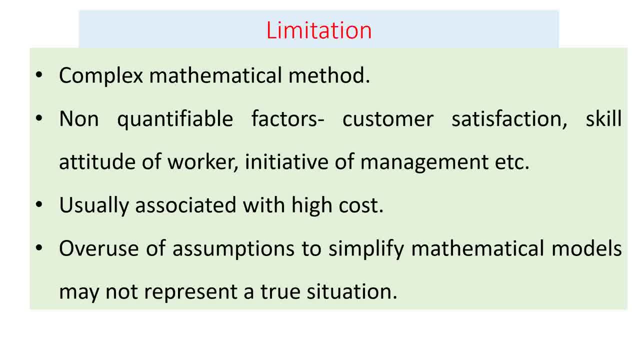 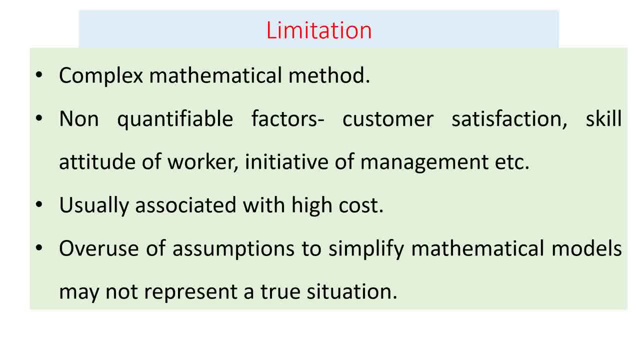 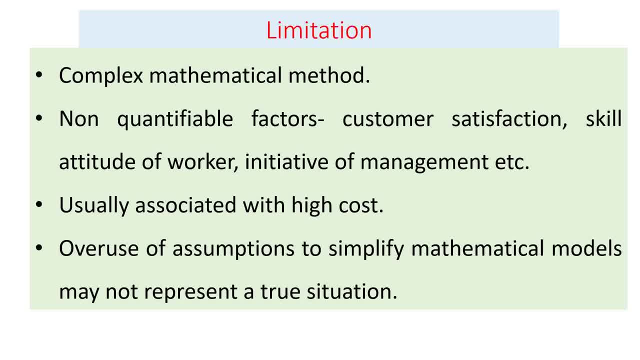 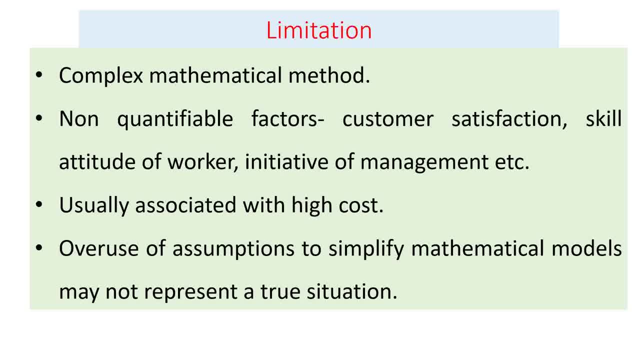 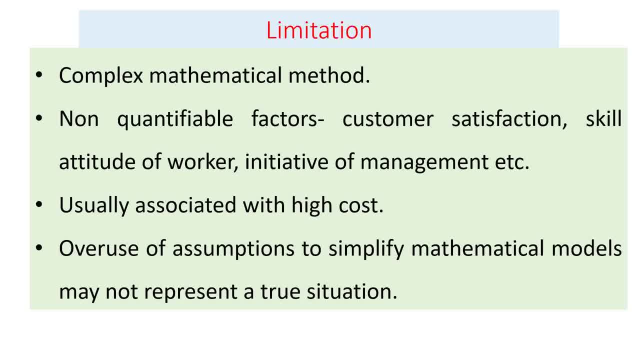 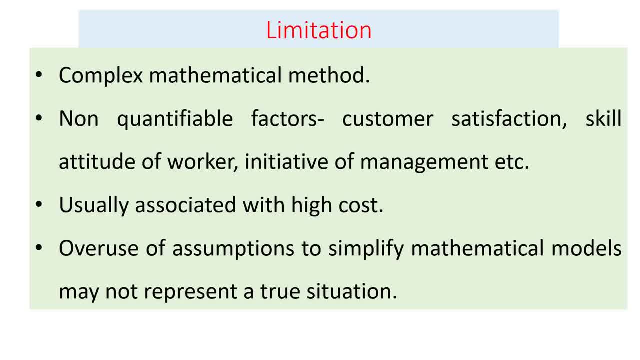 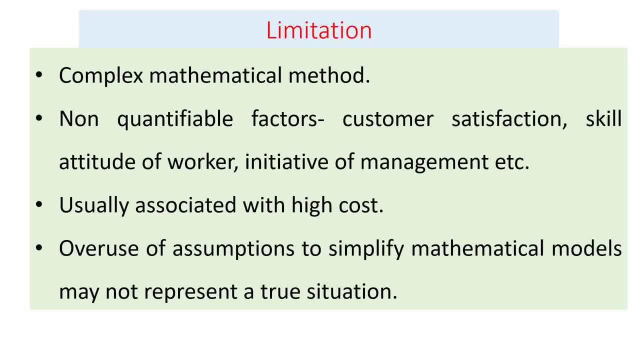 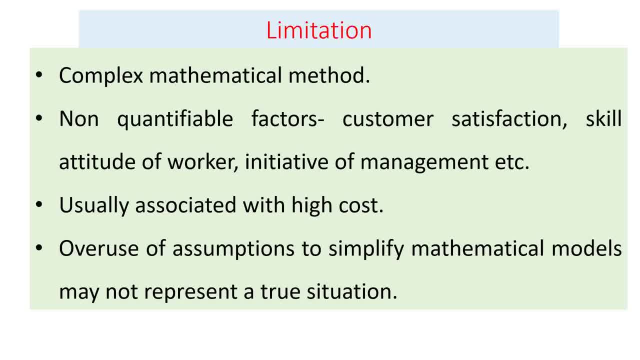 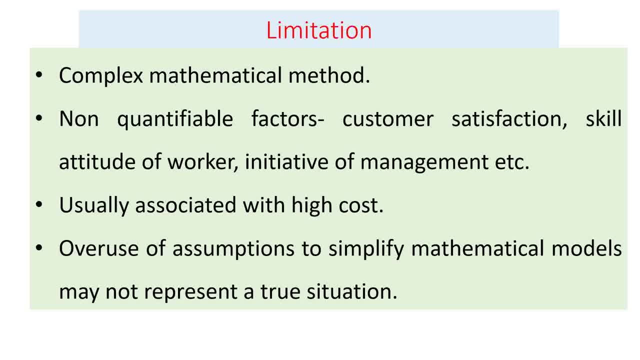 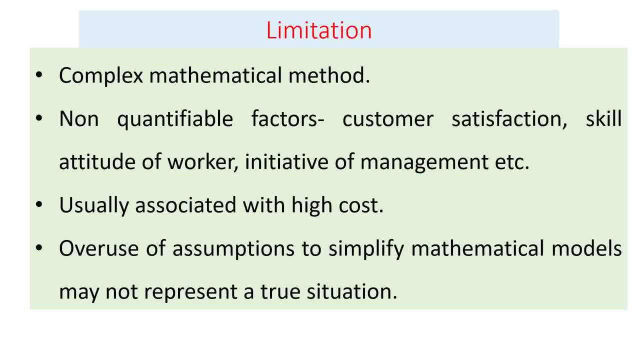 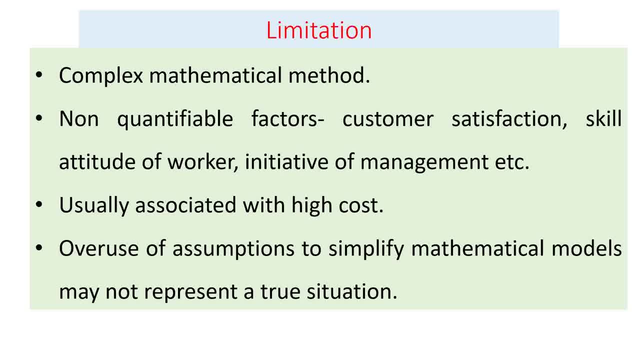 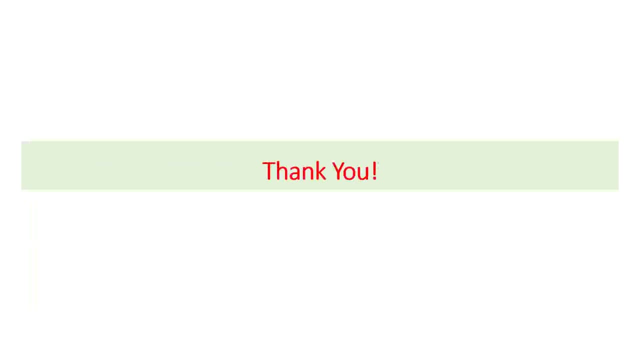 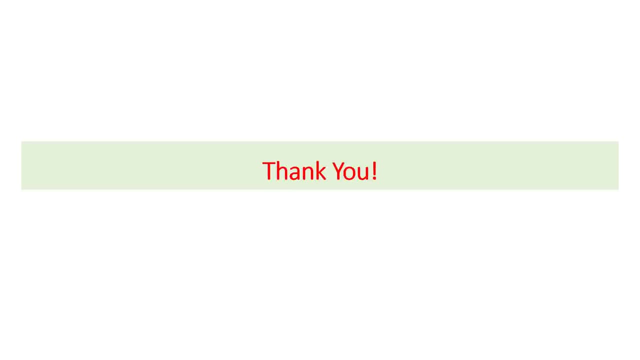 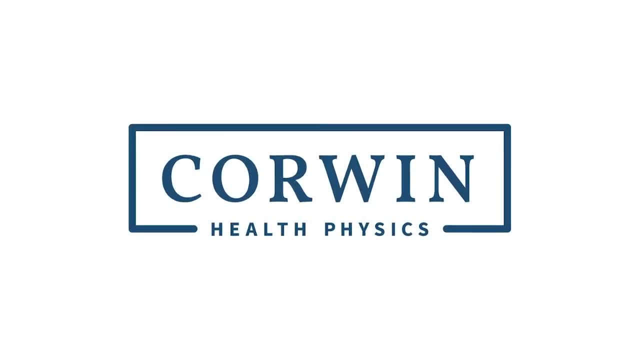 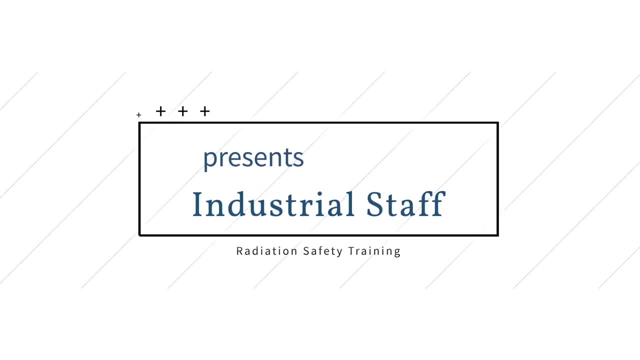 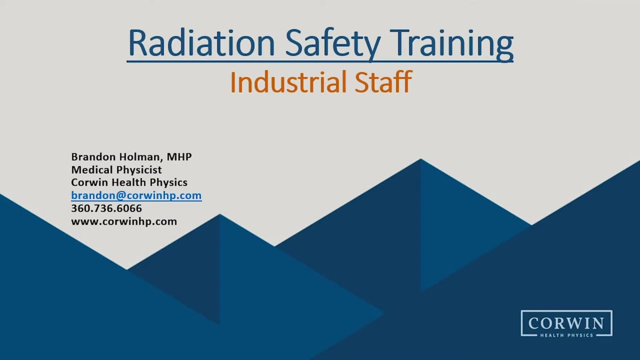 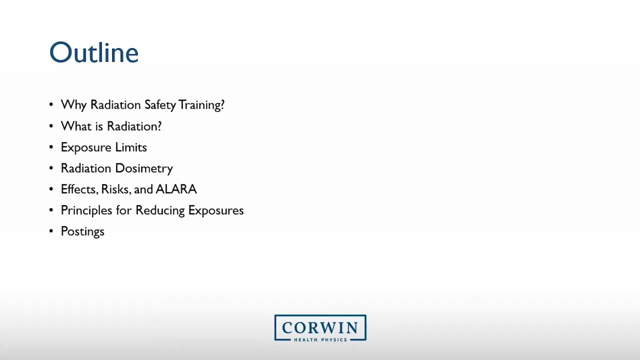 Hello, my name is Brandon Holman and this is Radiation Safety Training provided by Corwin Health Physics. This Radiation Safety Training is intended for those that work with or around analytical and industrial X-ray producing equipment. Before we get started, here is a review of what I will be discussing in this training. 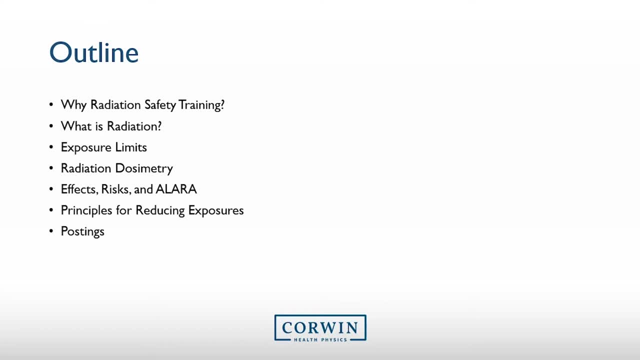 I will mainly be focusing on what exactly is radiation and the effects and risks associated with radiation exposure. I will go over principles that individuals use to reduce their exposure, but know that the machine you utilize takes care of these principles for you. And finally, I will end with important and required postings you should have around your department.